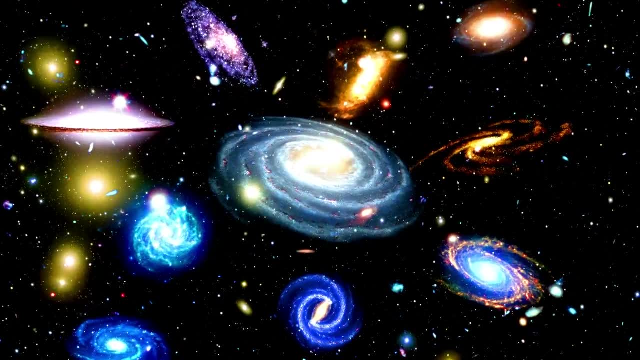 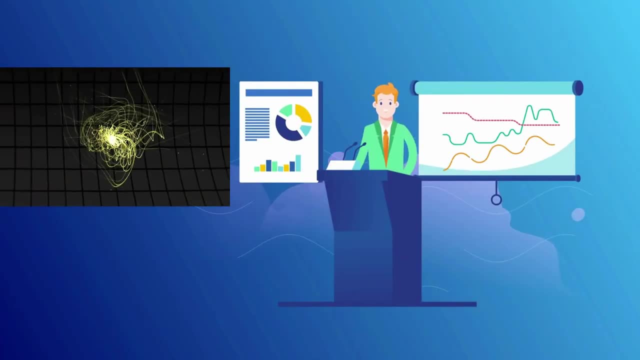 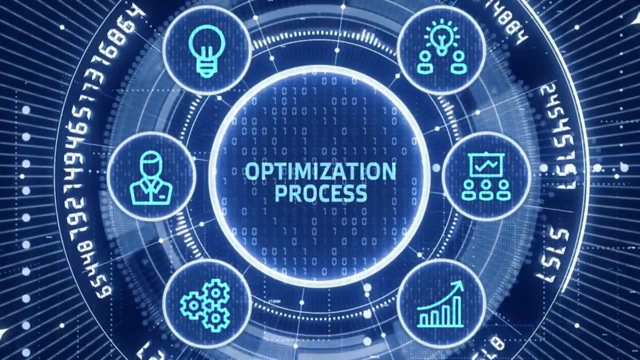 to create you, me and everything in the universe. From the earliest theories of matter to the cutting-edge discoveries of modern physics, scientists have relentlessly pursued the secrets of these elementary particles. By decoding their properties and interactions, we gain a deeper understanding of the universe and unlock the door to technological advancements that were once. 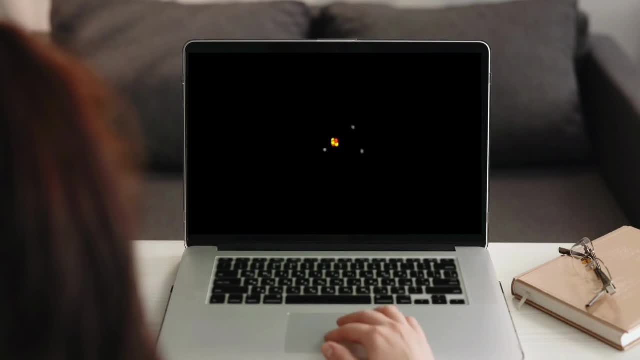 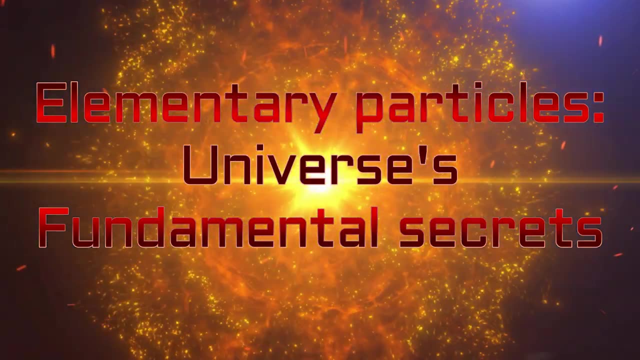 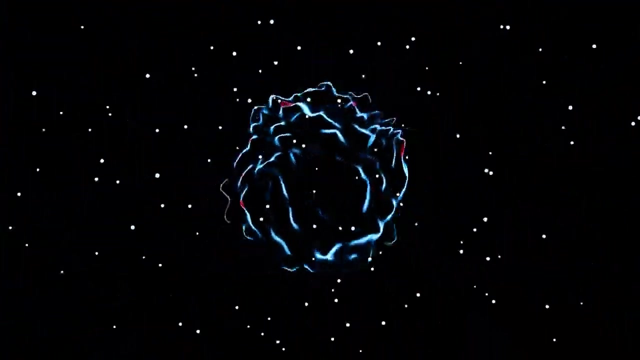 unimaginable. In this video, we're going to get a detailed breakdown of elementary particles, So without wasting any time, let's jump right in. Elementary particles, also known as subatomic particles, are the fundamental constituents of matter and energy. They are the building blocks that make up atoms and all other particles in 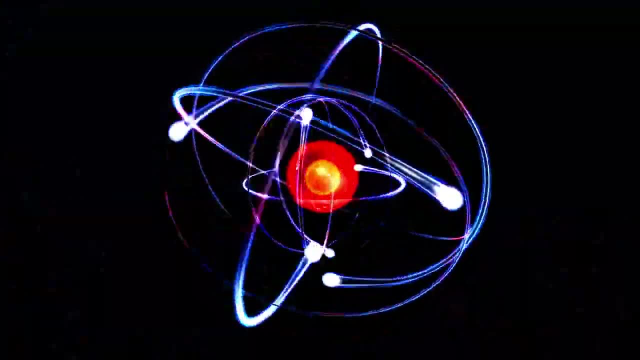 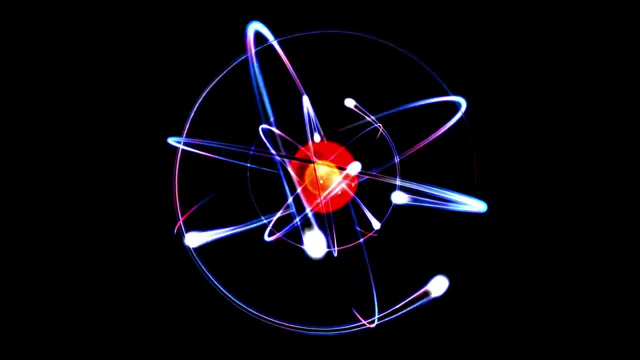 the universe. First let's explore some of the basic subatomic particles: electrons. Electrons are negatively charged particles that orbit the nucleus of an atom. They have a very small mass compared to protons and neutrons and are considered almost massless. 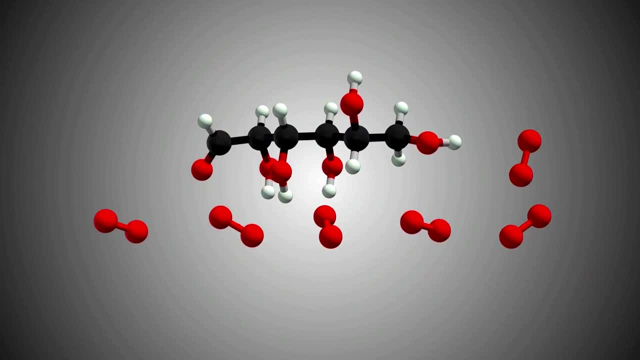 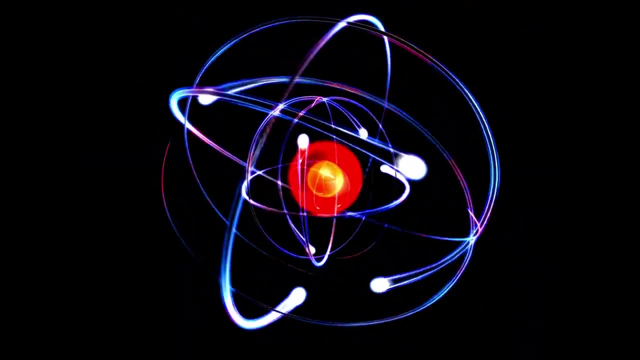 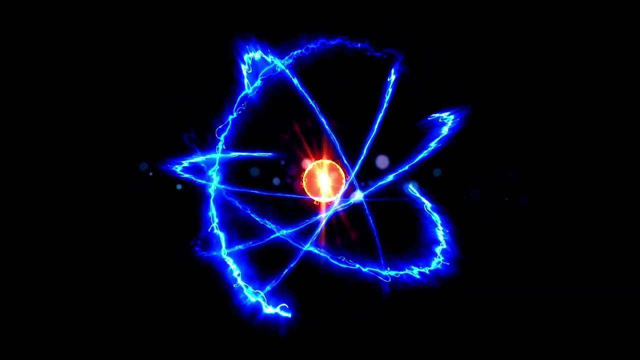 Electrons are crucial for chemical reactions and the formation of chemical bonds- Protons. Protons are positively charged particles found in the nucleus of an atom. They have a mass approximately 1,836 times greater than an electron. Protons carry a positive electrical charge that balances the negative charge of electrons. 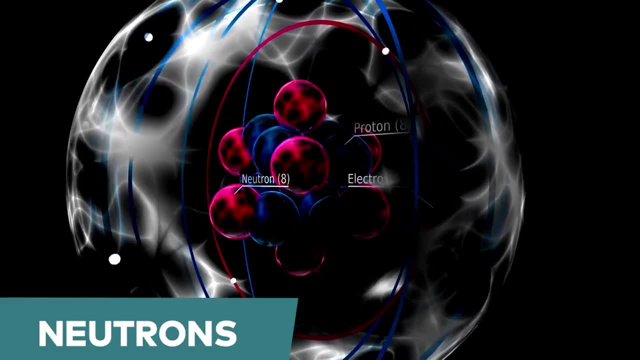 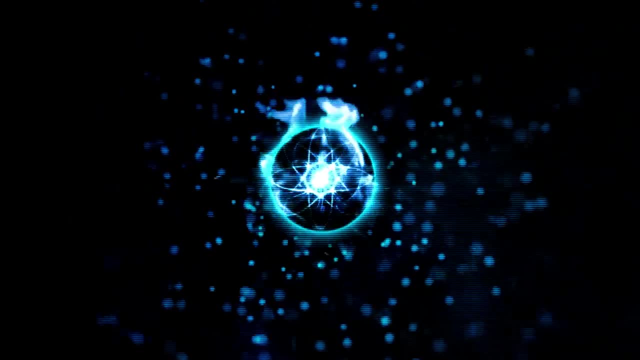 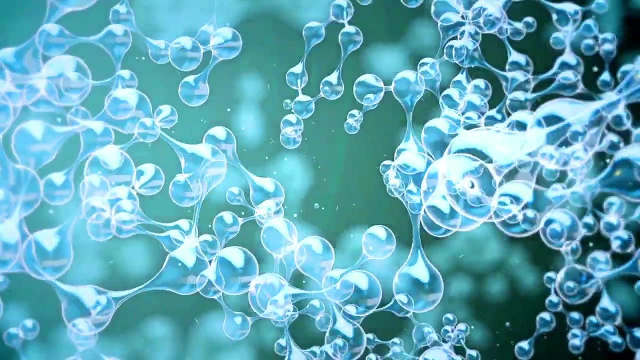 making atoms electrically neutral, And just like anything in the world of nuclear science, neutrons are electrically neutral particles also located in the nucleus of an atom. They have a mass similar to protons, making them collectively referred to as nucleons. Neutrons play a crucial role in stabilizing atomic nuclei by counteracting the electromagnetic 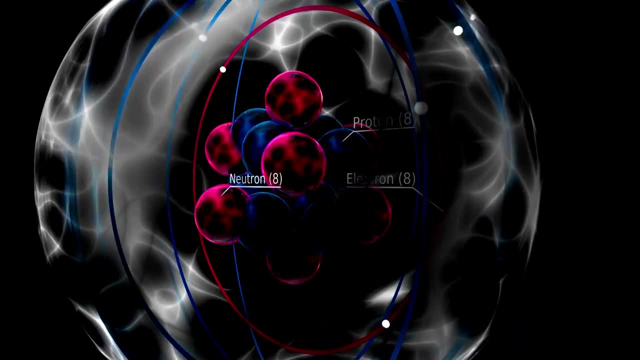 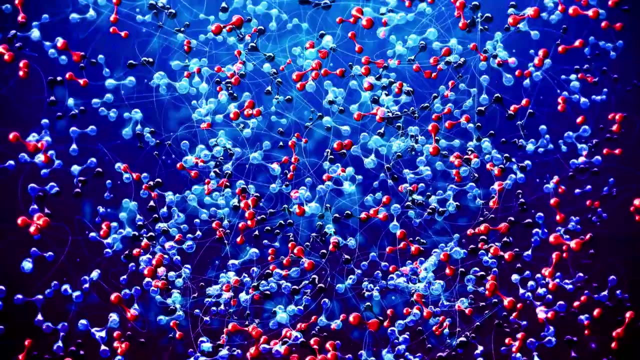 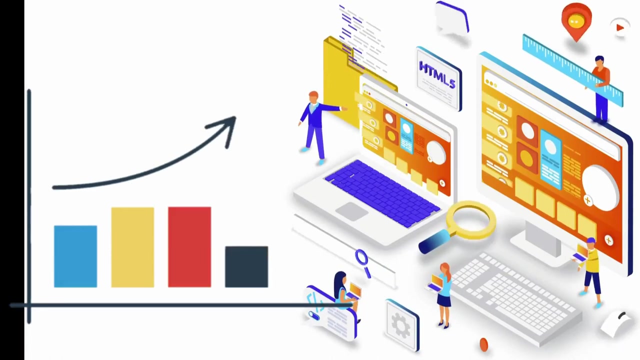 repulsion between protons. These three particles- electrons, protons and neutrons- form the basic structure of an atom. However, scientists have discovered numerous other subatomic particles with different properties and roles. The field of subatomic particles has experienced significant 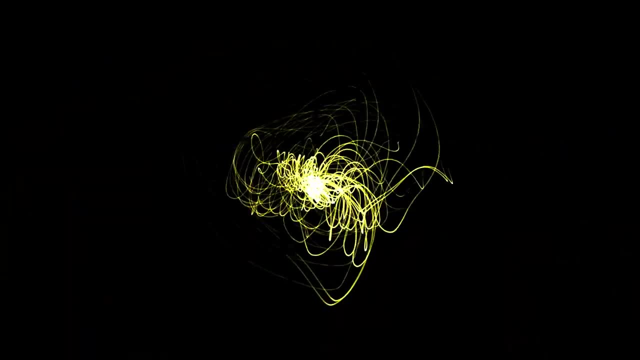 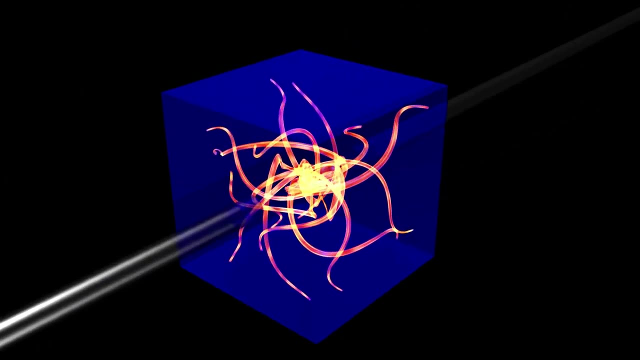 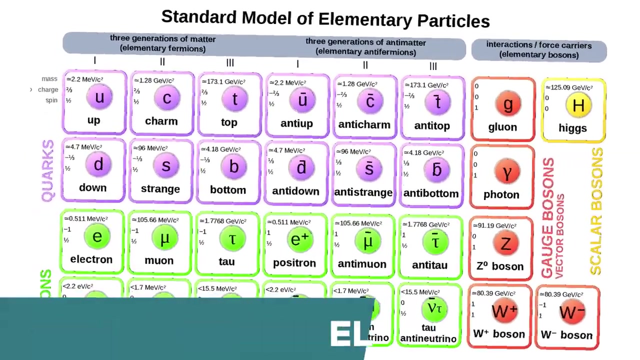 expansion and advancement, particularly with the development of powerful particle accelerators designed to investigate high-energy collisions involving electrons, protons and other particles interacting with matter. Within this field, the current understanding is organized within a framework called the Standard Model. The Standard Model is a conceptual framework that classifies 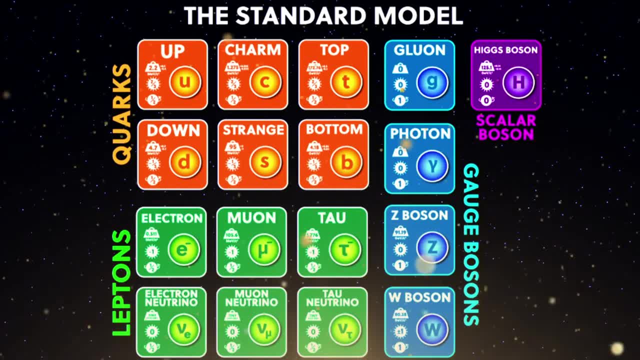 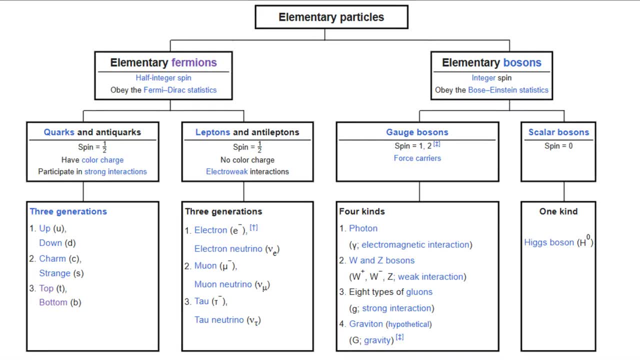 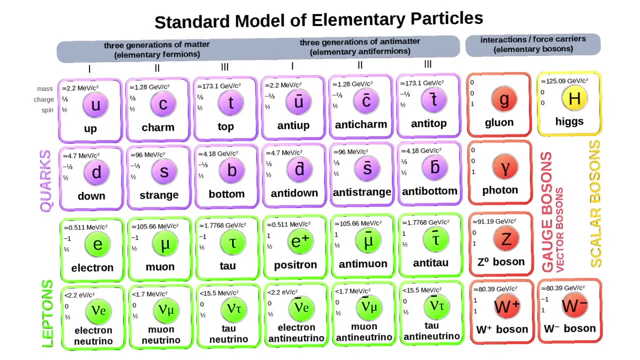 and describes all known subatomic particles based on theoretical models of the fundamental forces that govern matter. Let's take a look at this chart. Elementary particles are divided into elementary fermions and elementary bosons. All elementary particles are either bosons or fermions. The classification of elementary particles into bosons and fermions is based 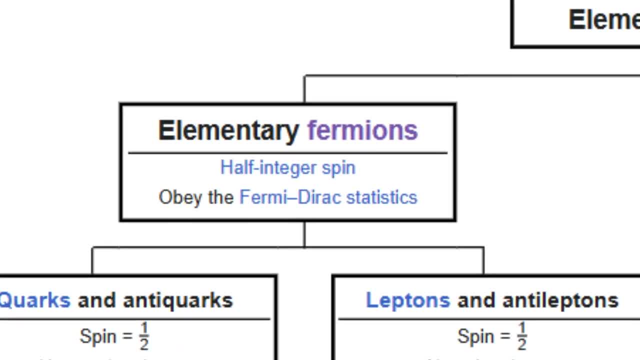 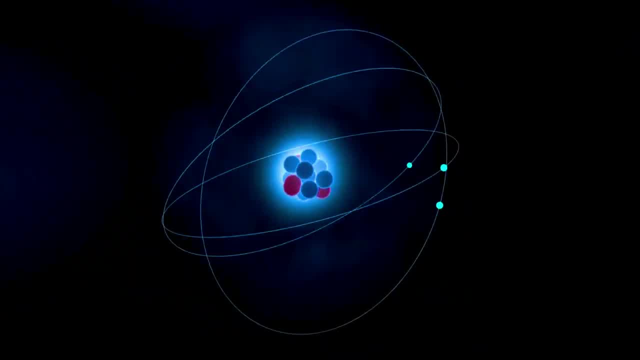 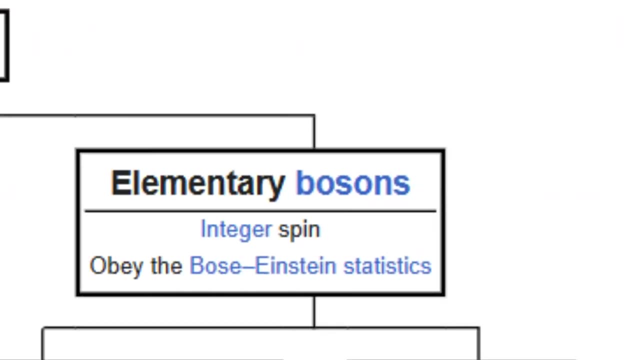 on their quantum statistics. Fermions adhere to Fermi-Dirac statistics, while bosons follow boson-Dirac statistics. Furthermore, their spin characteristics can be distinguished using the spin statistics theorem, with fermions having half-integer spins and bosons having integer spins. It is a quantum 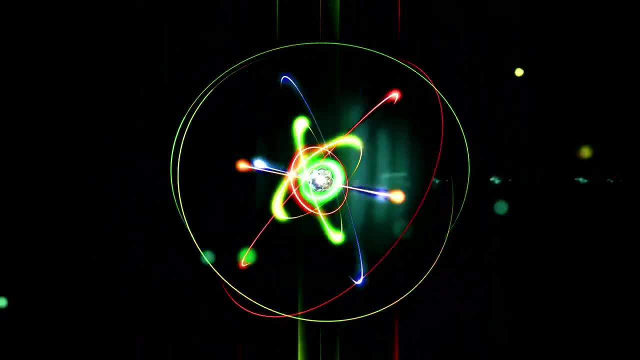 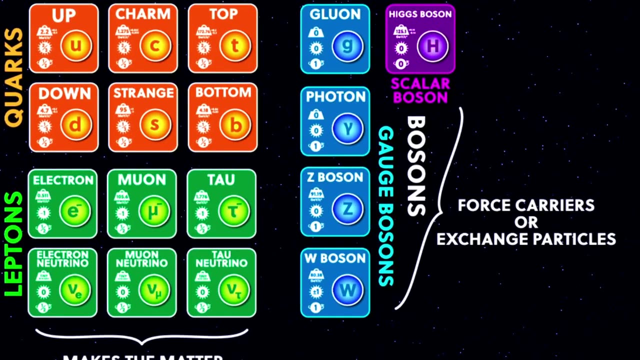 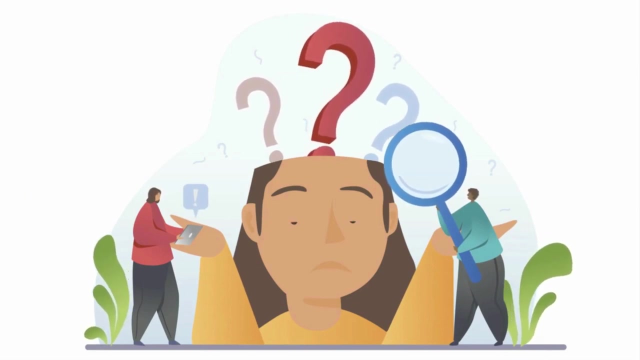 mechanical property and does not correspond to the actual spinning motion of the particles. Fermions are usually associated with matter, whereas bosons are generally considered force carrier particles. However, in the current state of particle physics, the distinction between the two concepts is unclear. 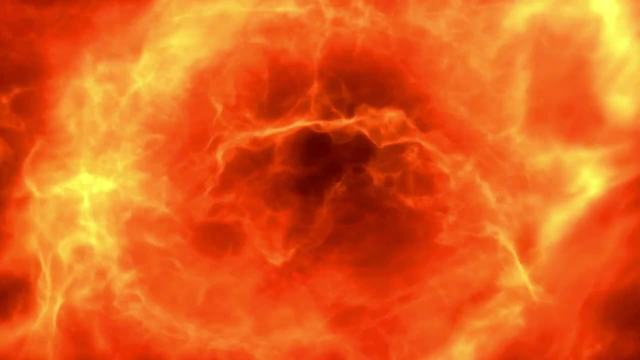 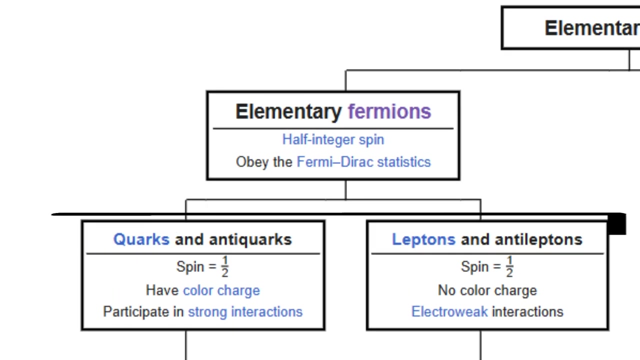 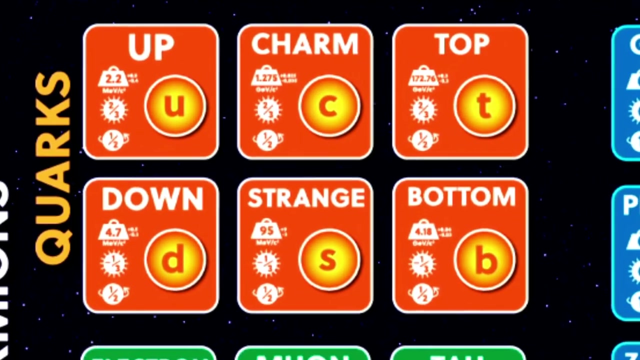 Weakly interacting fermions can also exhibit bosonic behavior under extreme conditions. Elementary fermions are divided into quarks and leptons, and both have corresponding antiparticles that are anti-quarks and anti-leptons. There are six types or flavors of quarks. 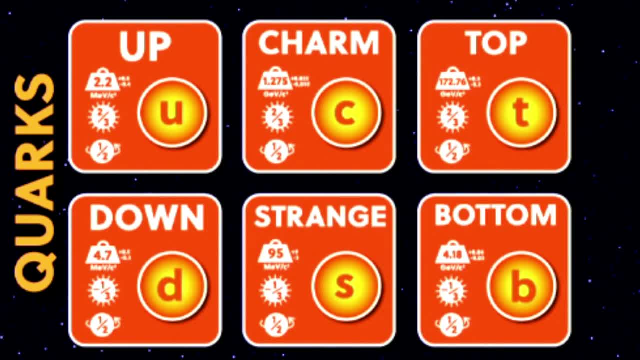 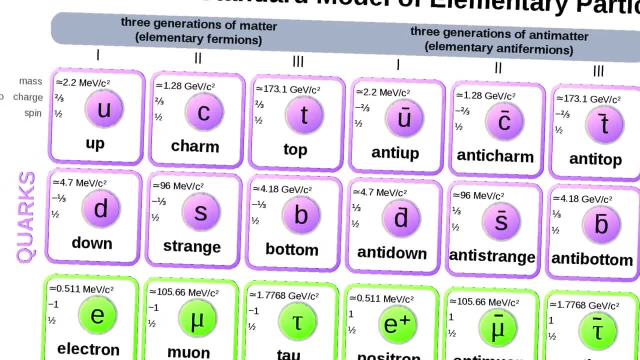 up, down, charm, strange top and bottom. For every quark type there is a corresponding type of antiparticle, known as an anti-quark. that differs from the quark only in that some of its properties, such as the electric charge, have equal magnitude but opposite signs. 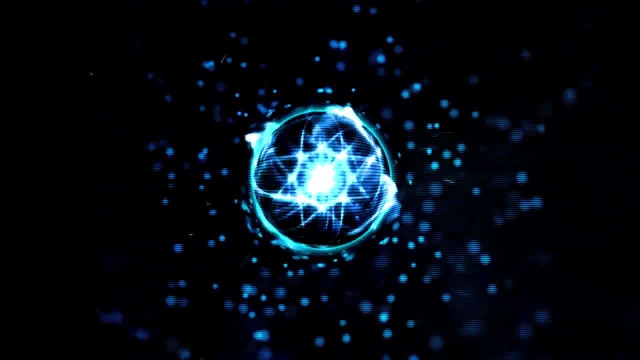 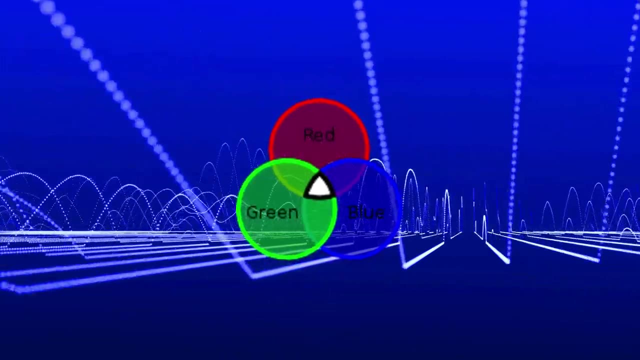 Quarks also have a property called color charge, which comes in three types: red, green and blue. It is important to highlight that these terms are just labels. Quarks are much smaller than the wavelength of visible light and do not have any color. 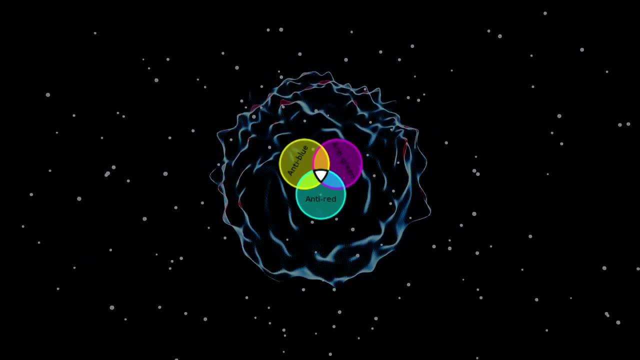 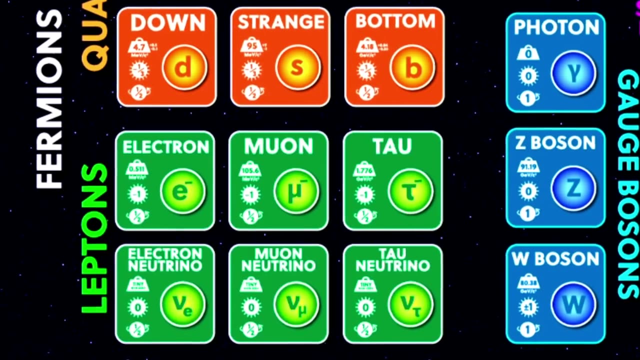 in the normal sense, Anti-quarks have the same color as their quarks but are represented as anti-red, anti-green and anti-blue. There are six types of leptons, grouped into three generations. The first generation leptons, also called electronic. 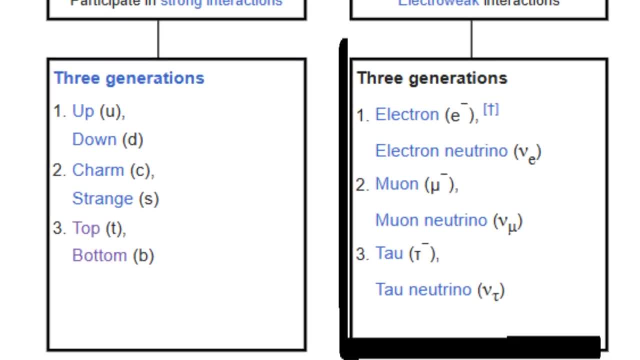 leptons comprise the electron and the electron neutrino. the second are the muonic leptons comprising the muon and the muon neutrino, and the third are the taonic leptons comprising the tau and the tau neutrino. For every lepton flavor there is a corresponding 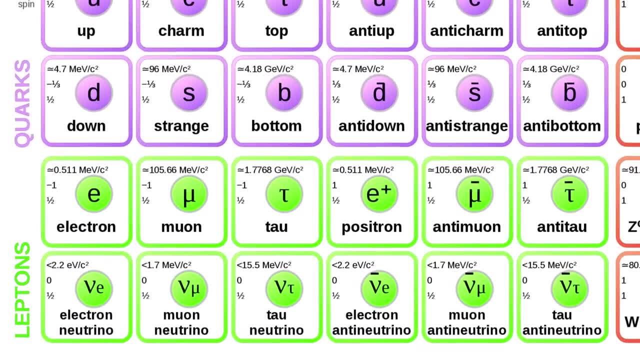 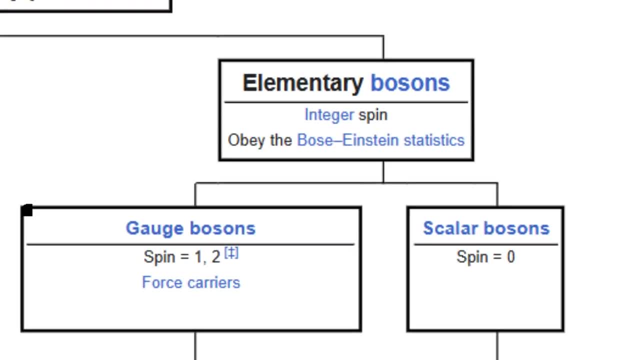 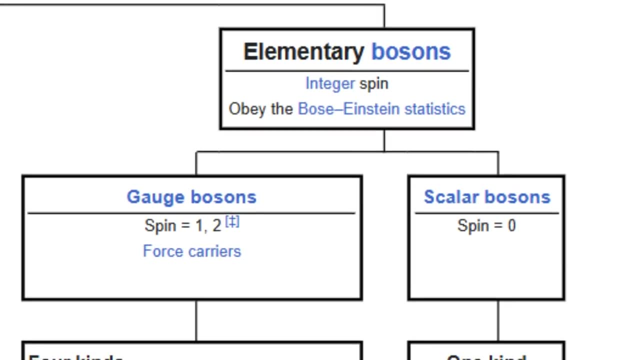 type of antiparticle known as an anti-lepton that differs from the lepton only in that some of its properties have equal magnitude but opposite sign. Elementary bosons are divided into gauge bosons and scalar bosons. Gauge bosons have spins of 1 and 2 and are associated with the following interactions: 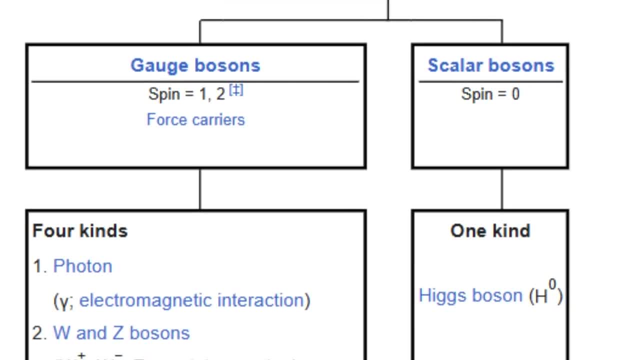 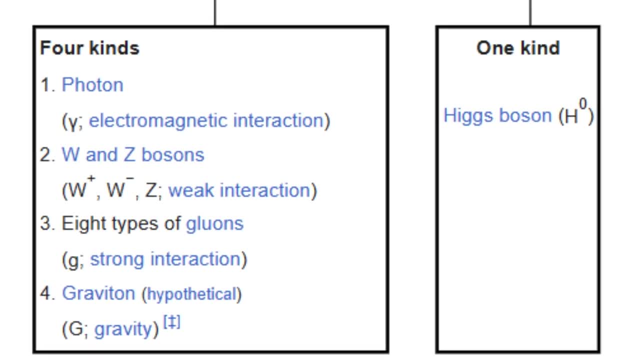 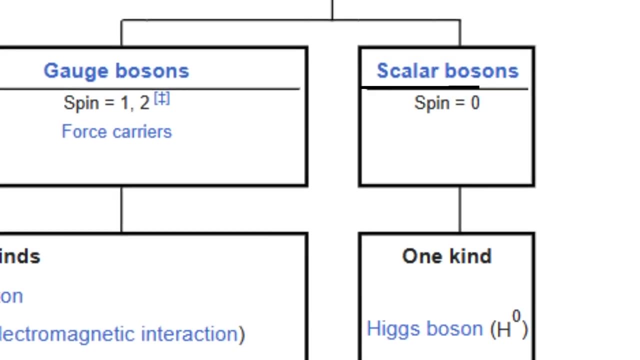 photons, electromagnetic interaction, W and Z bosons, weak interaction, gluons, strong interaction and the graviton, which is hypothetical and associated with gravity. Scalar bosons are a single kind, represented by the Higgs boson, and have a spin of 0.. 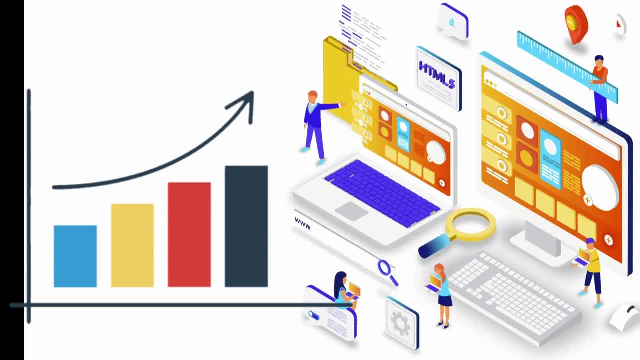 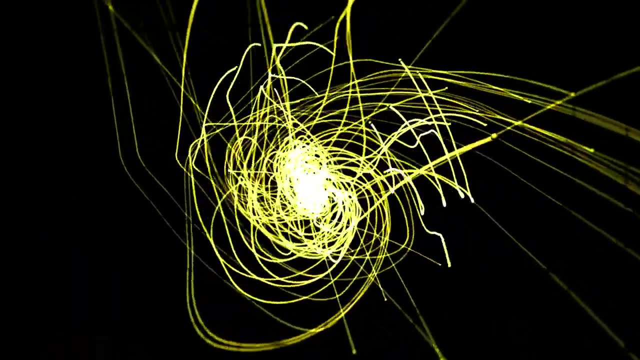 The development of particle physics was made possible in the 20th century with the advancement of increasingly sophisticated instruments capable of probing matter at extremely small scales, on the order of 10 to the power of negative 15 meters or less, that is, at distances comparable to the diameter of 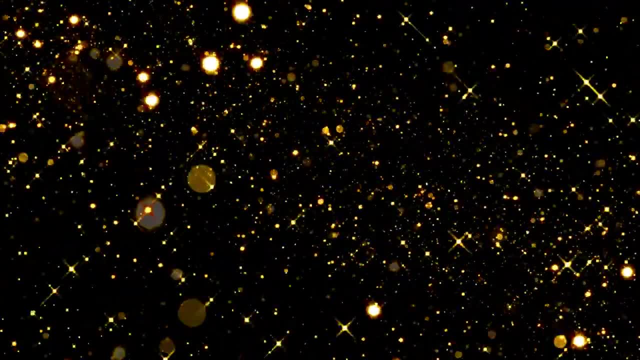 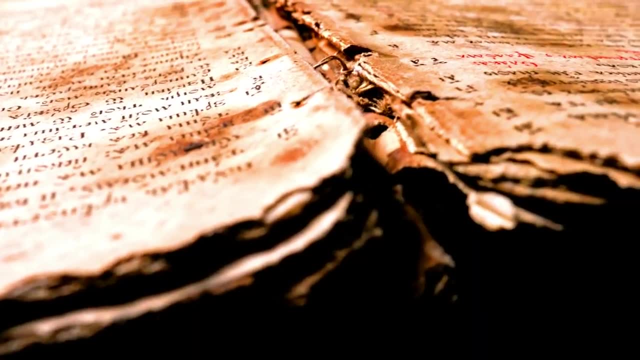 the proton or neutron. However, the foundational concepts and philosophy of particle physics can be traced back much further to ancient Greece, around 500 BCE. During that time, the Greek philosopher Leucippus and his student Democritus proposed the concept of particle physics as a 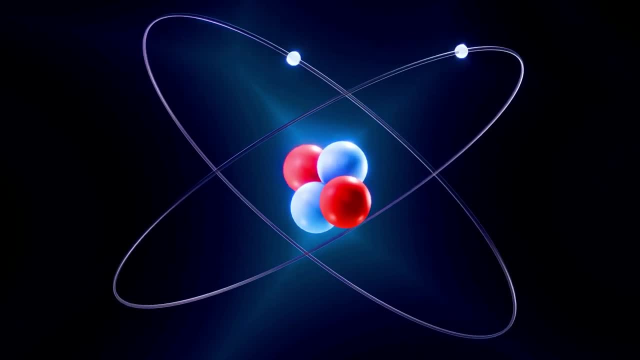 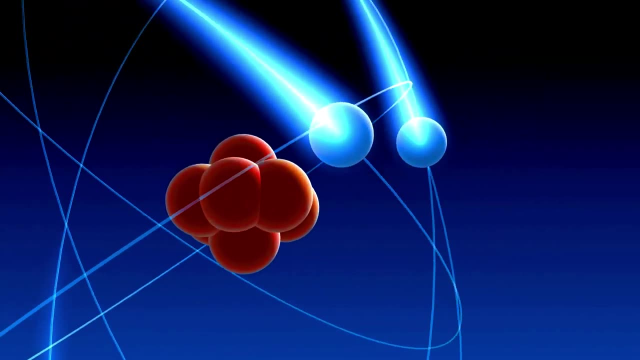 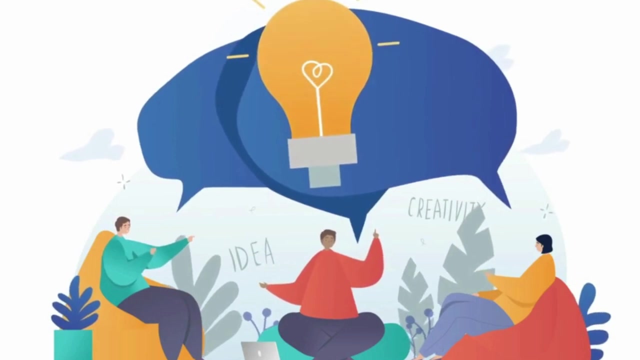 concept that matter is composed of tiny, indivisible particles called atoms. These early atomists hypothesized that atoms were the fundamental building blocks of all matter and were invisible to the naked eye. Despite the groundbreaking nature of their ideas, the concept of atoms was largely neglected for over 2000 years. Instead, the prevailing view- 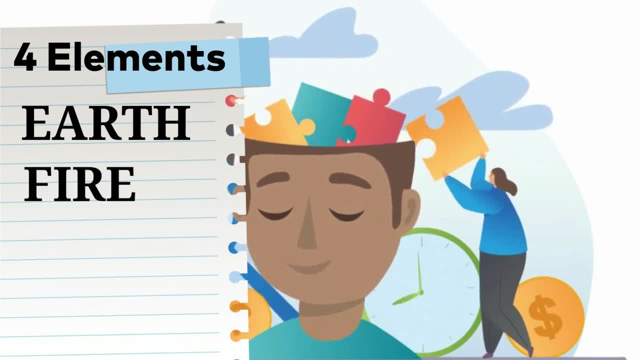 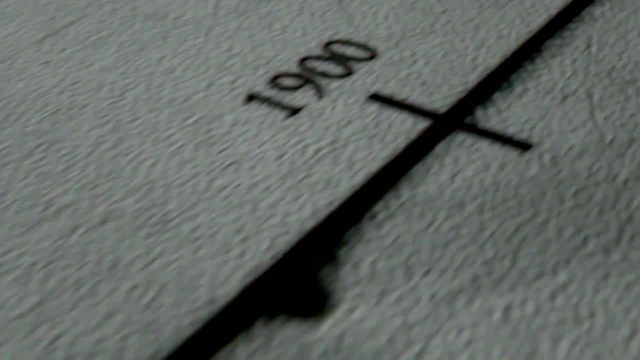 held that matter was made up of four elements: earth, fire, air and water. However, by the beginning of the 19th century, the atomic theory of matter had experienced a resurgence in popularity. The work of British chemist and physicist. 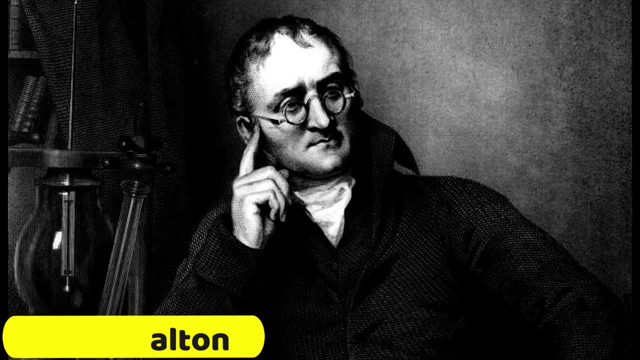 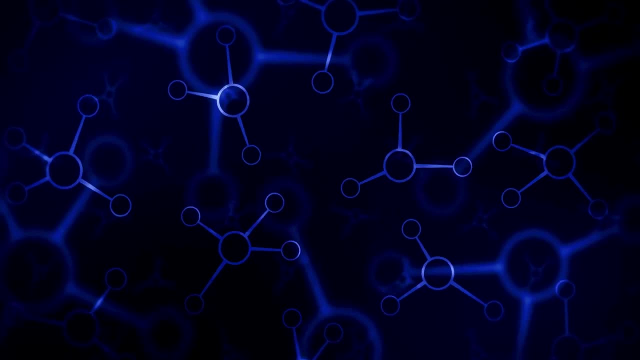 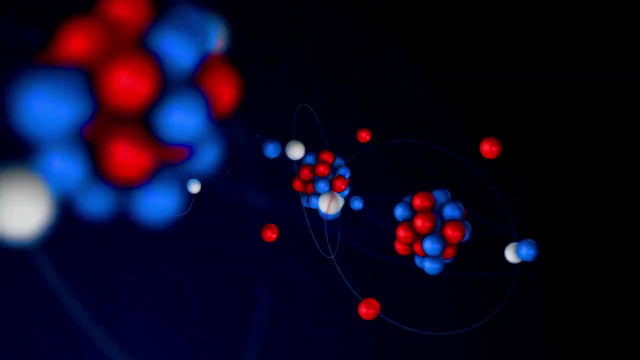 John Dalton played a significant role in strengthening atomic theory. Dalton's studies suggested that each chemical element is composed of its own distinct type of atom. His atomic model proposed that atoms were indivisible and had specific properties that determined the behavior of different elements. Dalton's atomic theory. 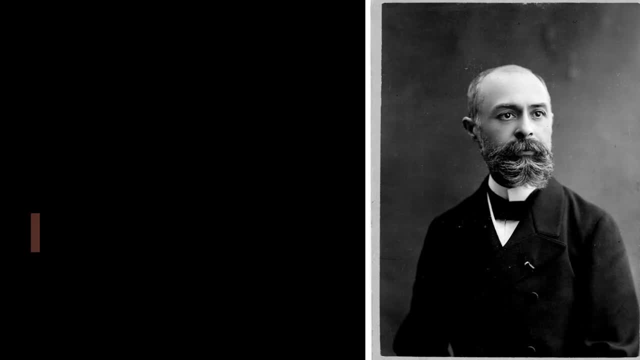 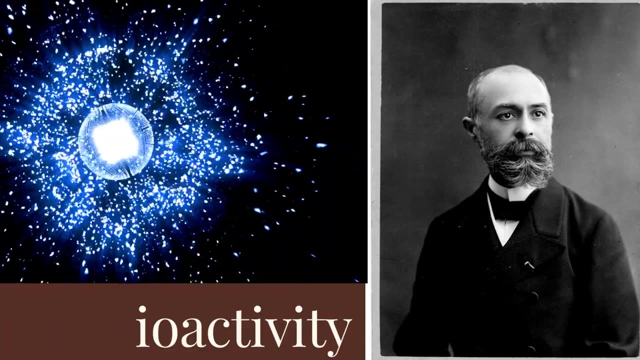 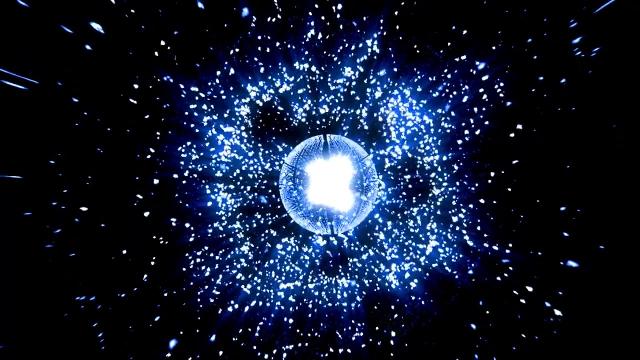 formed the basis for the modern understanding of atoms. In 1896, Henri Becquerel, a French physicist, made the landmark discovery of radioactivity. He found that certain materials emitted radiation spontaneously, without any external influence. This discovery opened up a new field of study and challenged the prevailing notion of atoms as immutable and indivisible. 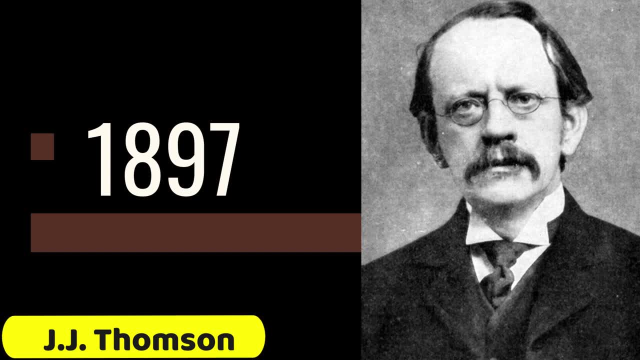 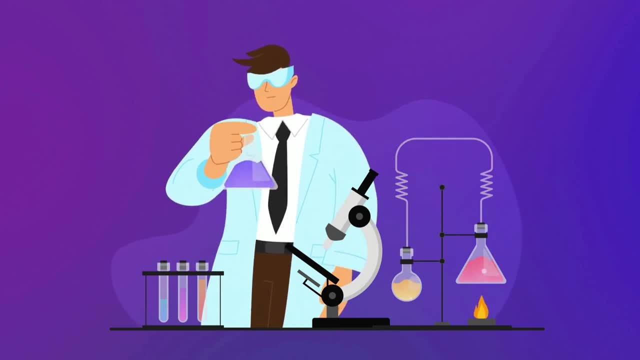 In the subsequent year, JJ Thomson, a physicist at the University of Cambridge in England, conducted experiments that provided evidence for the existence of subatomic particles. Thomson's experiments involved investigating the potential of atoms, the presence of atoms in the atmosphere and the presence of radioactivity. The 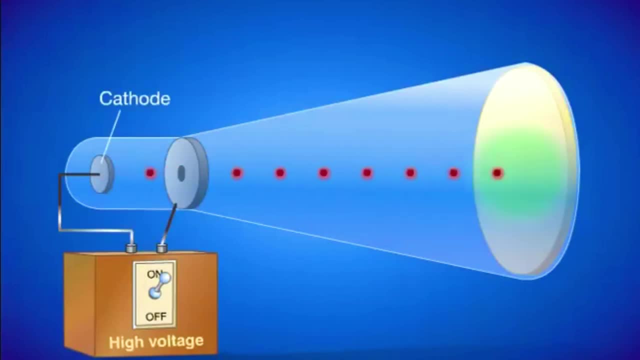 properties of cathode rays, which are streams of electrons emitted from a negatively charged electrode in a vacuum tube. By measuring the deflection of cathode rays in electric and magnetic fields, Thomson determined that they were negatively charged particles with a much smaller mass than that of hydrogen, the lightest known atom at the time. This groundbreaking discovery- 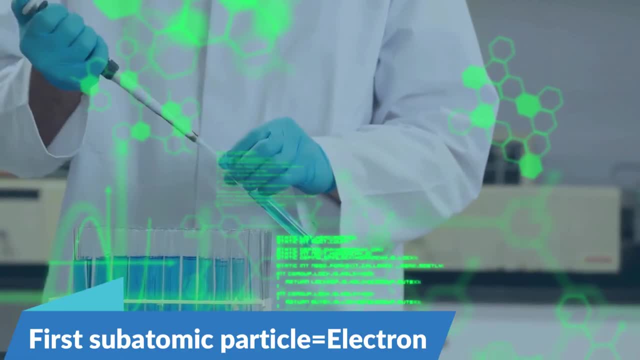 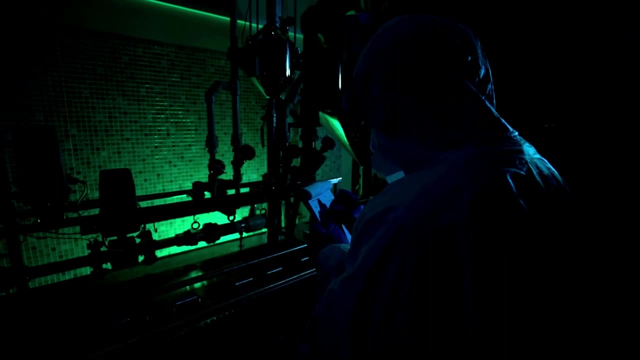 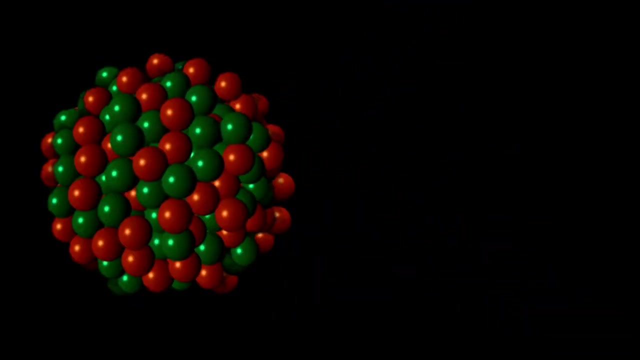 revealed the existence of the first subatomic particle, the electron. Building upon these advancements, Ernest Rutherford and Frederick Soddy, while working at McGill University in Montreal, made significant contributions to the understanding of radioactivity and atomic transmutation. In 1902, they observed that certain radioactive elements decayed over time. 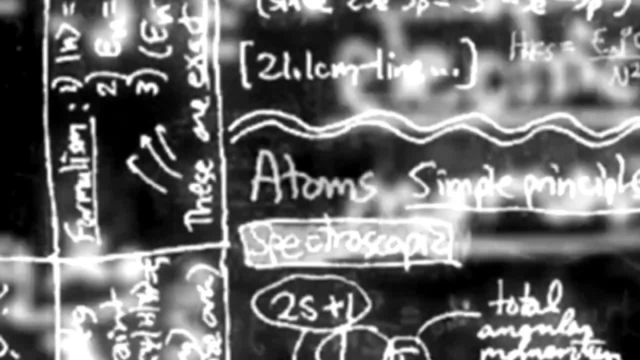 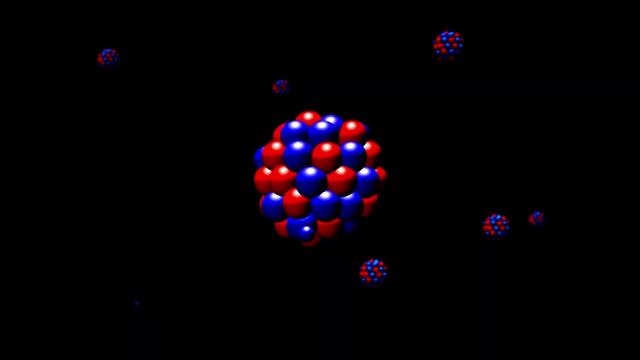 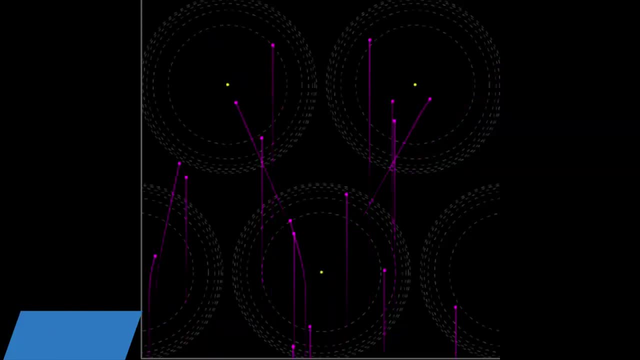 transforming into atoms of different elements. This discovery shattered the idea of atoms as immutable and indivisible entities, providing clear evidence that atoms can change and transmute into different types of atoms. In 1911, Ernest Rutherford conducted an experiment known as the Gold Foil Experiment, which provided crucial insights into the 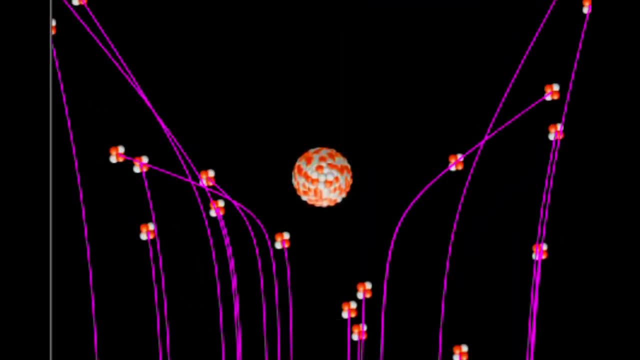 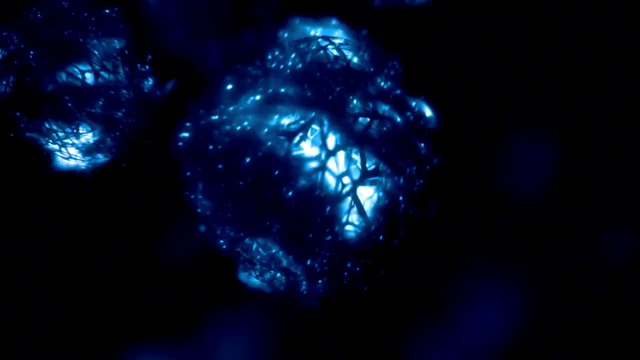 structure of the atom. He discovered that most of the mass of an atom is concentrated in a tiny, dense nucleus at the center. This revelation challenged the previously held idea of the atom as a uniform and indivisible entity. Rutherford proposed a new model for the atom, likening it to 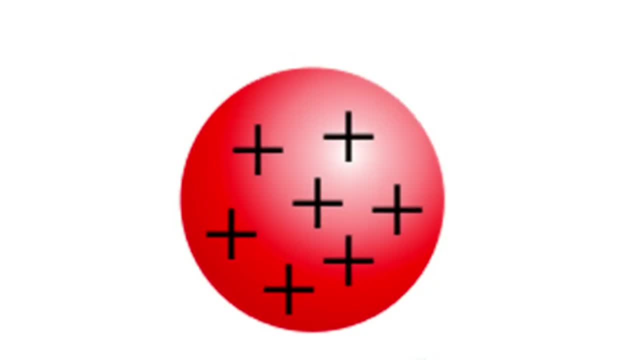 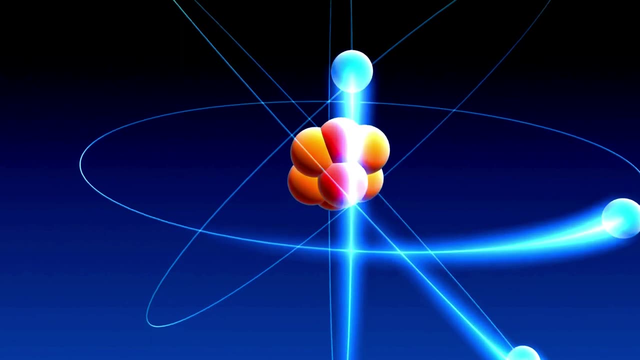 a miniature solar system. According to his model, the negatively charged electrons orbited around the positively charged nucleus, much like planets orbiting the sun. This concept of electron orbits explained how the atom remained stable despite the electron's energy. The atom remained stable despite 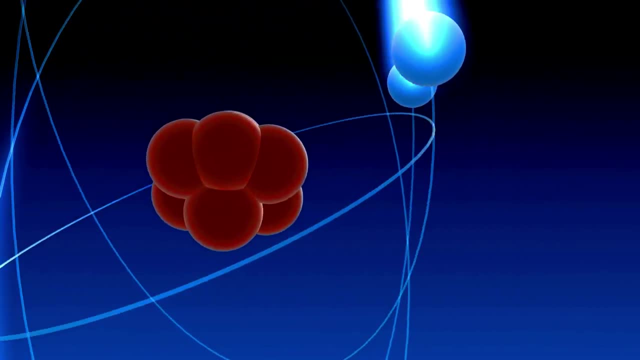 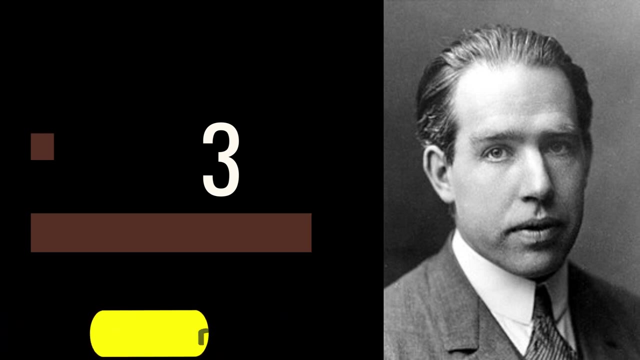 the electrostatic attraction between the positively charged nucleus and the negatively charged electrons. Niels Bohr, a Danish theorist, further refined the atomic model in 1913 by incorporating the concept of quantization, which had been introduced by German theoretical physicist Max. 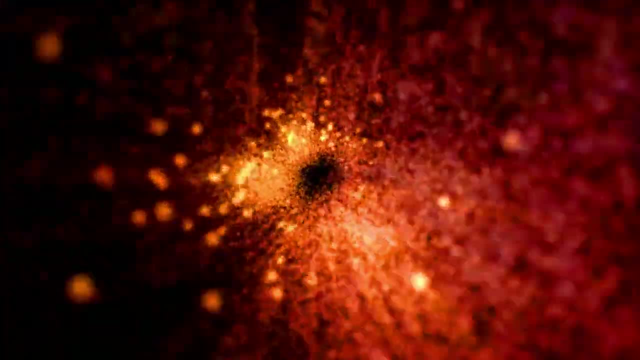 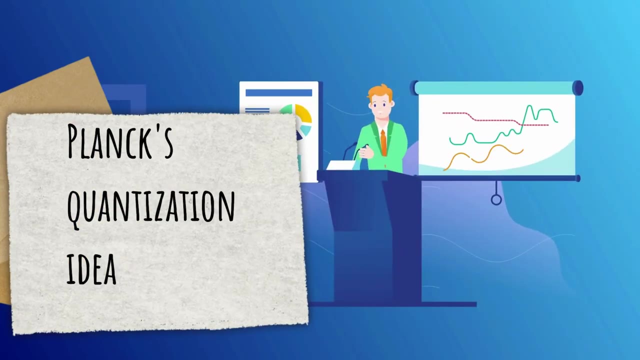 Planck. Planck's work demonstrated that electromagnetic radiation, including light, occurs in discrete packets of energy called quanta or photons. Building on Planck's quantization idea, Bohr postulated that electrons orbit the atom and that electrons orbit the. 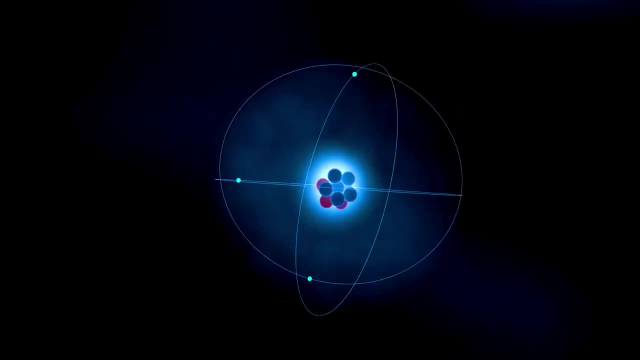 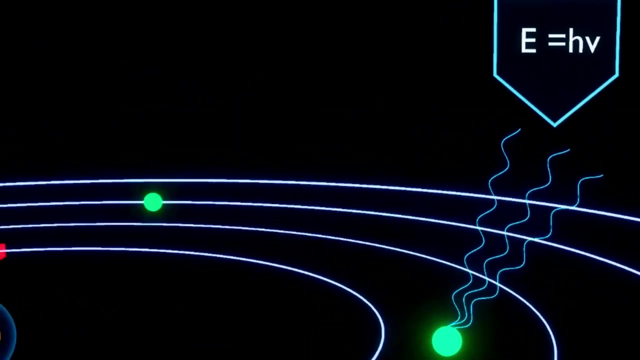 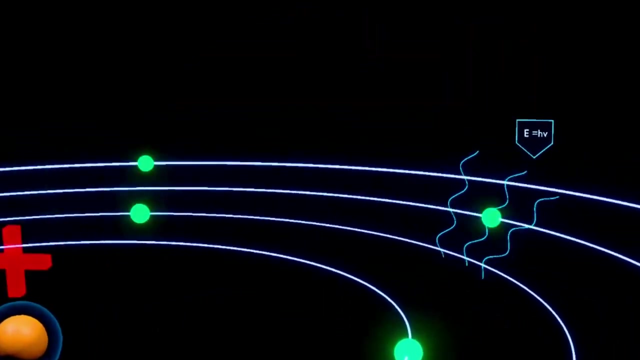 nucleus in fixed orbits or energy levels. Each orbit has a specific size and energy, and electrons can transition between these orbits by either emitting or absorbing quanta of energy. This theory provided a framework for understanding the stability of atoms and the emission and absorption of light at specific wavelengths. This concept helped explain various atomic 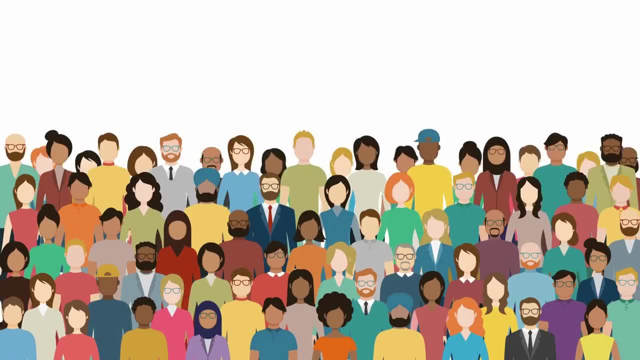 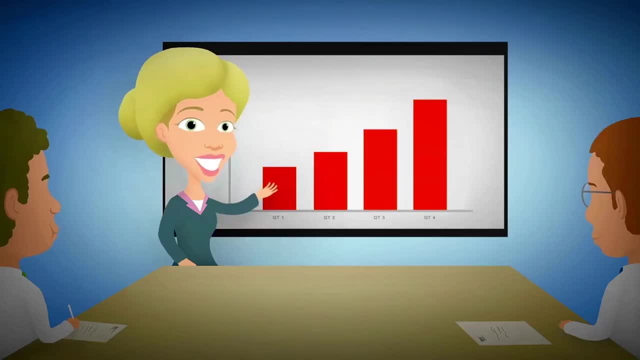 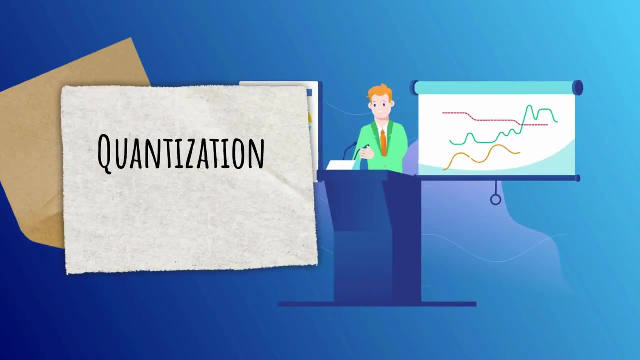 and subatomic phenomena and gained wider acceptance in the scientific community. This understanding laid the groundwork for further advancements in the field of particle physics, leading to the development of more sophisticated models and theories to describe the behavior of subatomic particles and their interactions. The concept of quantization, which emerged in the 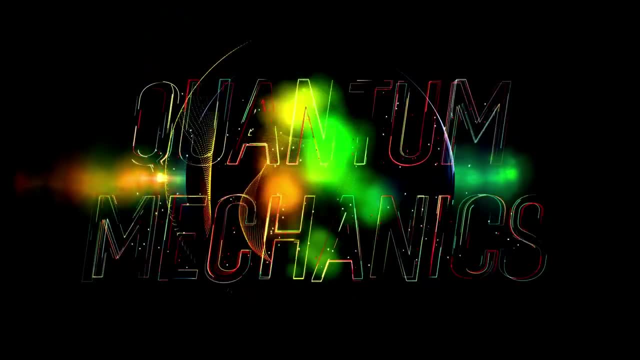 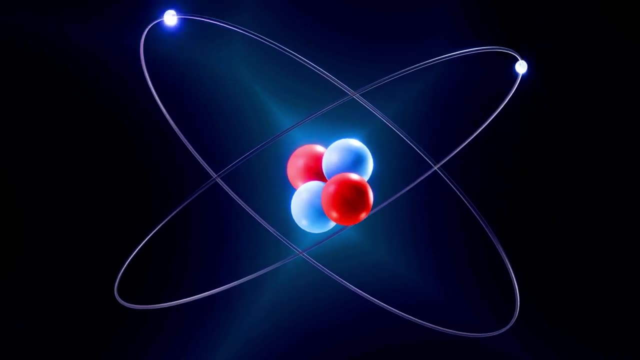 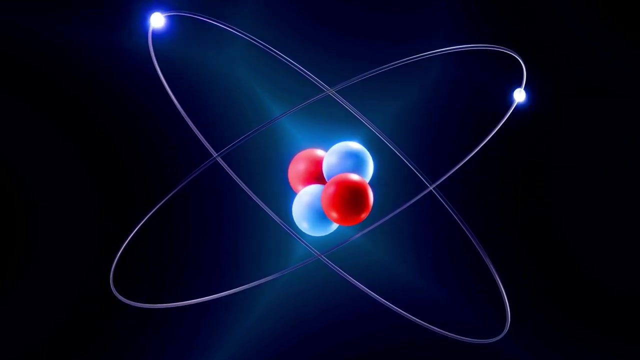 early 20th century led to the development of quantum mechanics and provided a successful framework for understanding the structure of atoms. Niels Bohr's model proposed that electrons and atoms move only in specific orbits characterized by fixed values of angular momentum, each associated with a quantum number that takes integer values. However, in the 1920s, 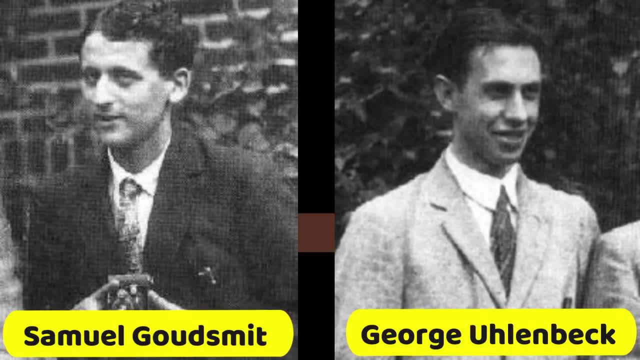 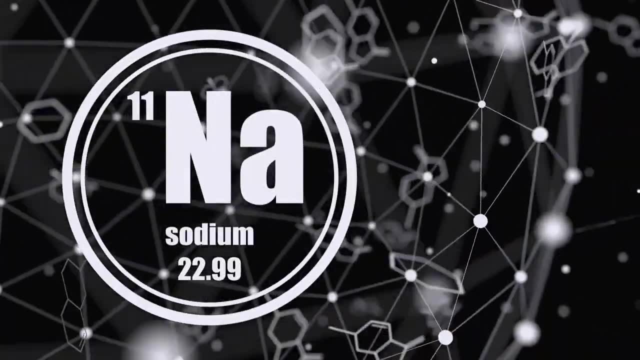 Gaude-Smith and George Uhlenbeck, Dutch physicists, recognized that a fourth quantum number was necessary to fully explain the spectral properties of alkali metal atoms, such as sodium, which have one outer valence- electron- beyond the main core. Gaude-Smith and Uhlenbeck introduced the idea of 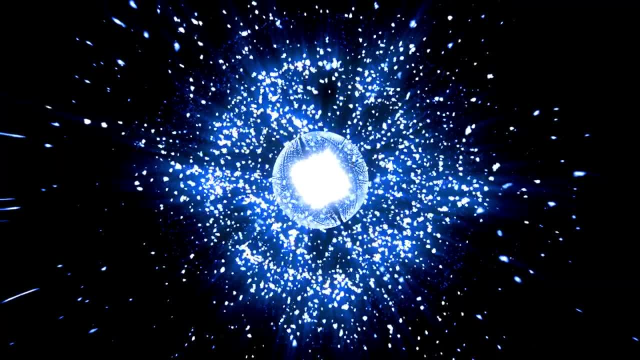 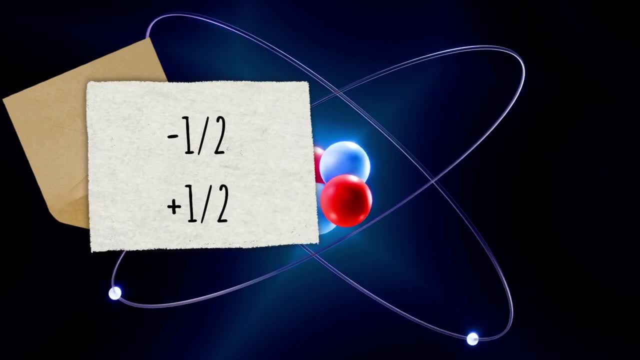 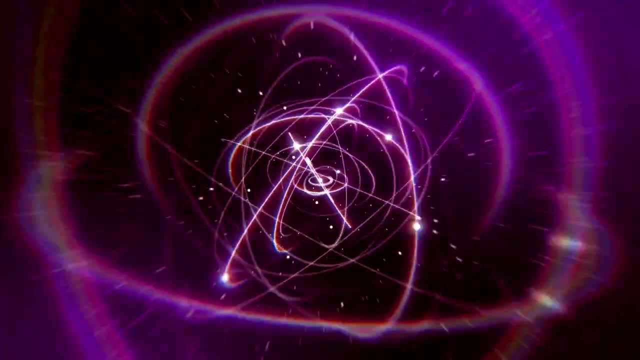 an internal angular momentum, or spin, associated with electrons. They suggested that electrons possess a spin quantum number that can have two possible values, minus one half and plus one half. This spin corresponds to the rotation of the electron as if it were a spinning electric charge. It implies that each electron 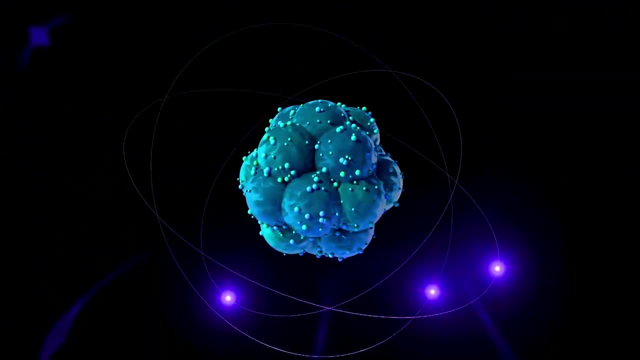 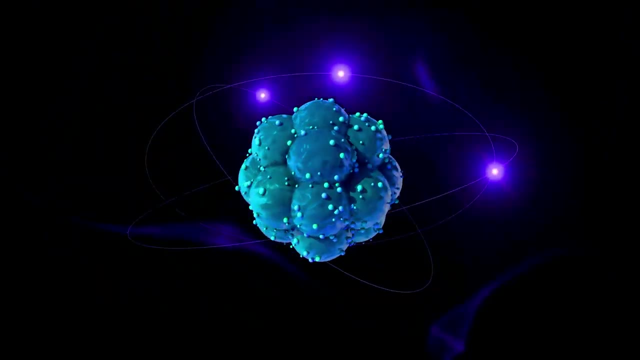 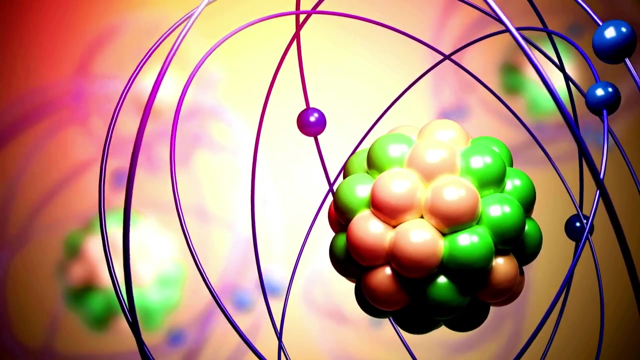 generates its own magnetic field and has a magnetic moment. The orientation of this internal magnet with respect to the magnetic field of the rest of the atom can be either parallel or anti-parallel, resulting in two quantized states and two possible values for the spin quantum number. Spin is now understood as an inherent property of all subatomic particles. 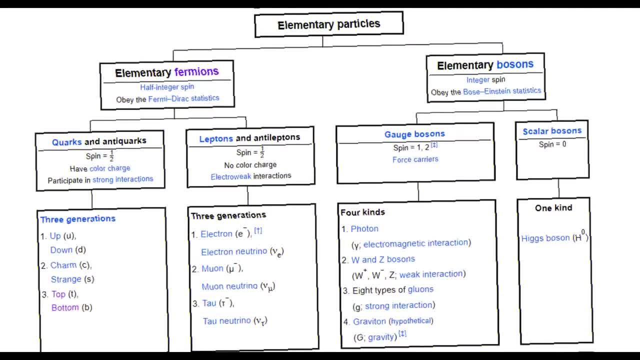 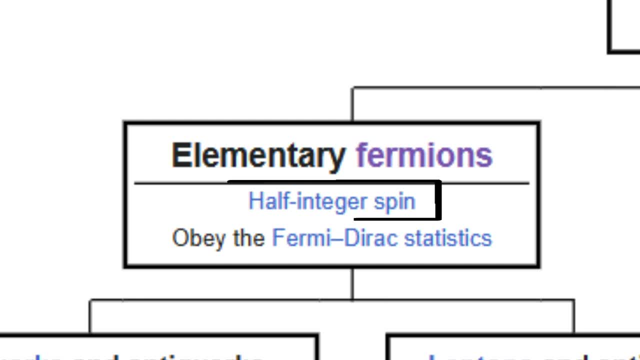 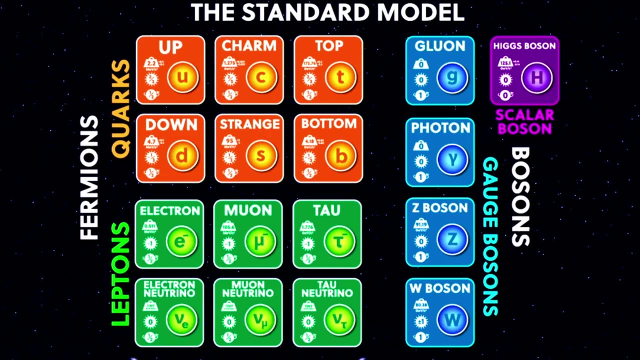 It is a fundamental characteristic used to classify particles into two main groups: fermions and bosons. Fermions have half integer values of spin, one, half, three, halves, etc. while bosons have integer values of spin zero, one, two, etc. In the standard model of particle. 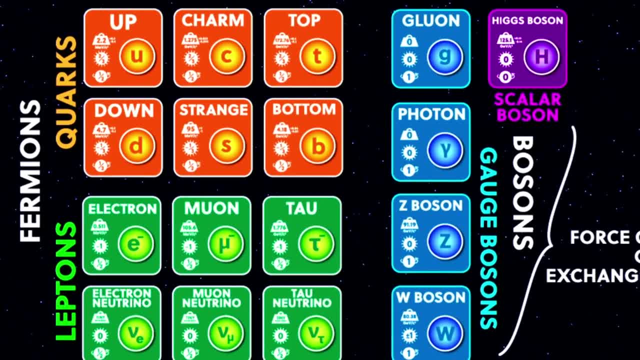 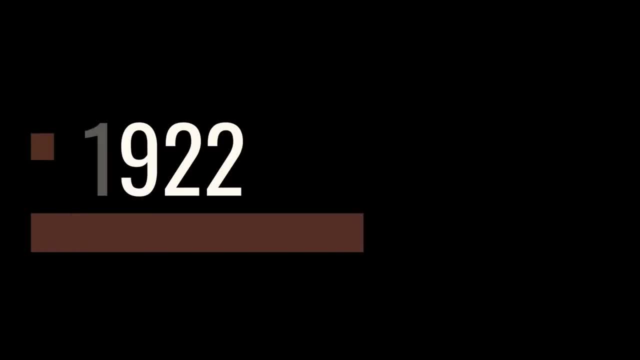 physics matter. particles such as quarks and leptons are fermions, while force-carrying particles like photons are bosons. Two years after the work of Gaude-Smith and Uhlenbeck, the English theorist Paul Dirac provided a sound theoretical background for the concept of electron. 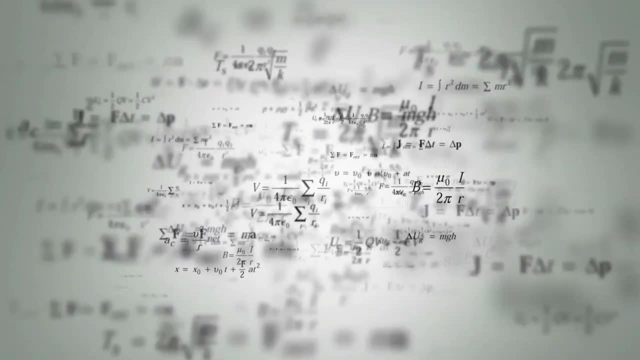 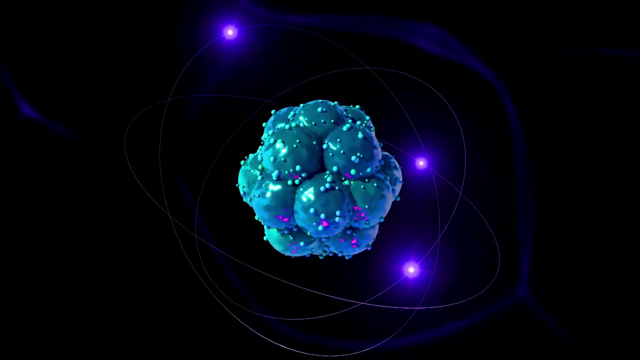 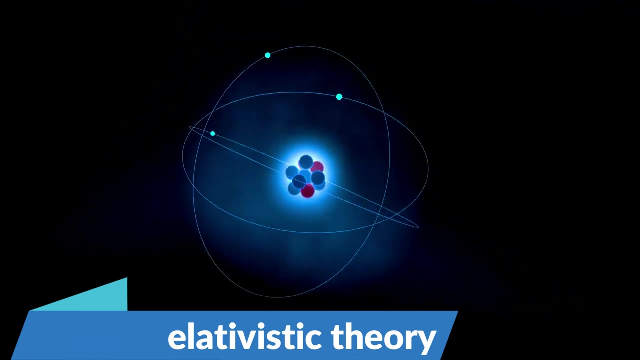 spin. In the development of quantum mechanics, Paul Dirac played a crucial role by incorporating Albert Einstein's theory of special relativity into the framework of quantum theory. His work provided a solid theoretical foundation for the concept of electron spin. Dirac's relativistic theory of the electron revealed that, in addition to its orbital 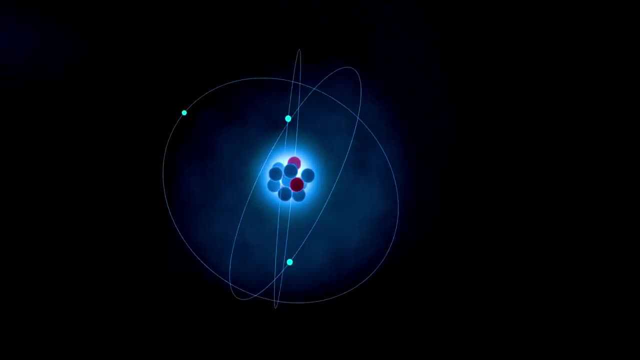 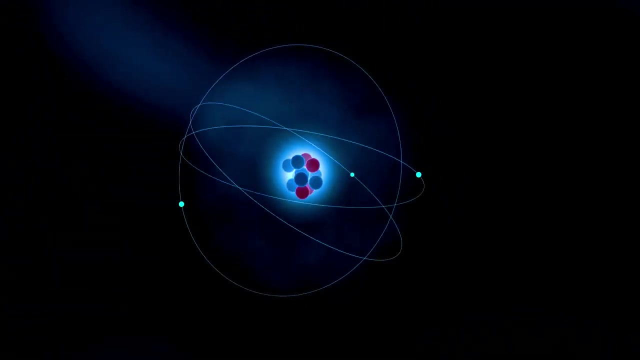 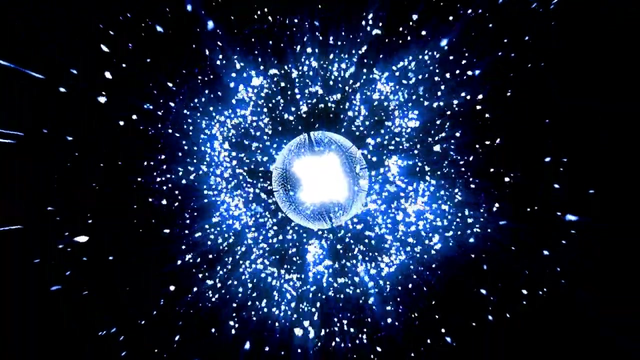 motion around the nucleus, the electron must possess an intrinsic angular momentum called spin. Spin is a quantum mechanical property that gives rise to the magnetic moment of the electron. When Dirac applied special relativity to the electron's behavior, he derived an equation that described the allowed energies of the electron. However, 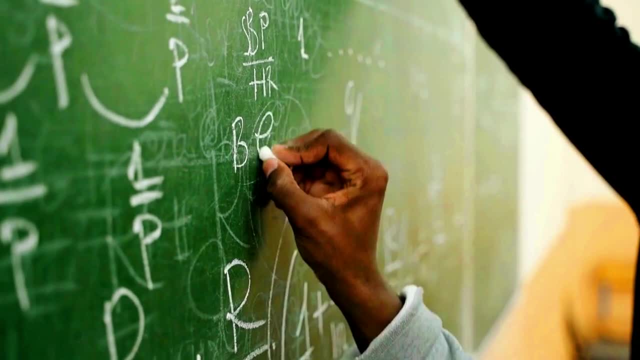 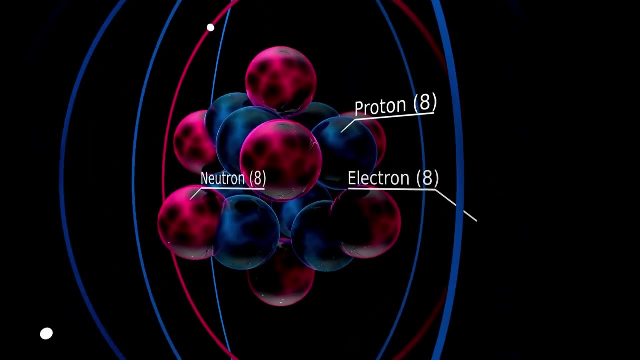 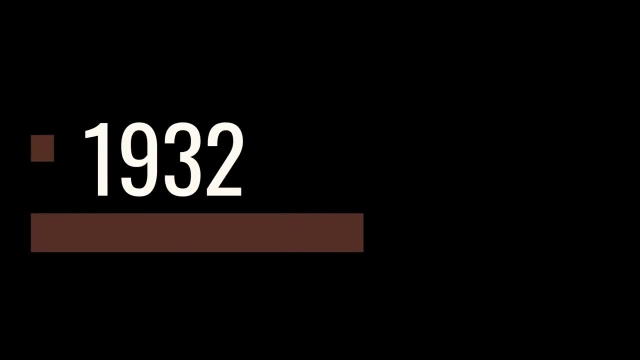 this equation had a peculiar feature: It had two solutions, a positive solution and a negative solution. The positive solution corresponded to what was already known as normal electrons, but the negative solution appeared to describe electrons with a positive charge, which seemed contradictory. In 1932, Carl Anderson made a significant discovery by 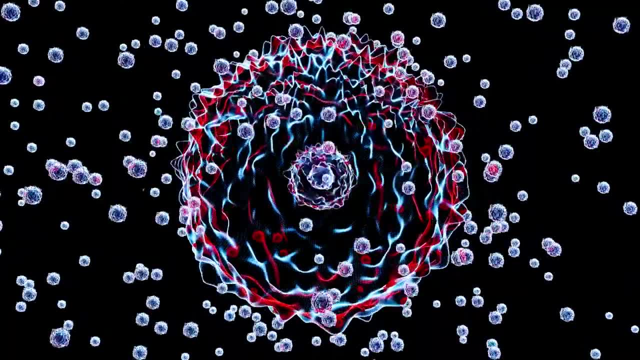 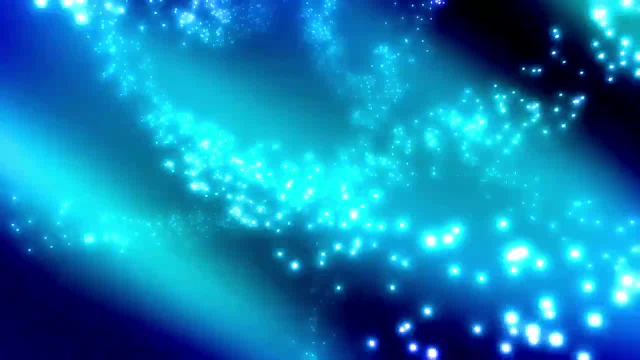 describing the particle known as the positron, which resolved the mystery surrounding the negative solutions in Dirac's equation. Positrons are very similar to electrons in terms of their mass and spin, but they possess the opposite electric charge. These positrons were the first. 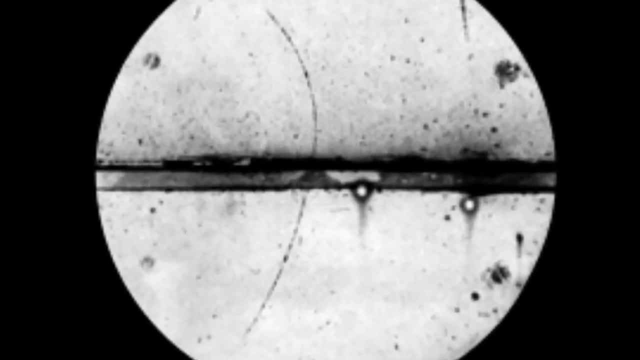 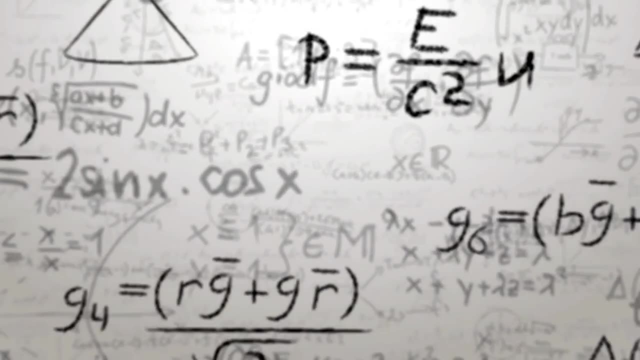 antiparticles to be experimentally observed, confirming Dirac's prediction. Dirac's theory, which incorporated special relativity in quantum mechanics, applies to all subatomic particles with a spin of one half. Consequently, all particles with this spin value are expected to have an 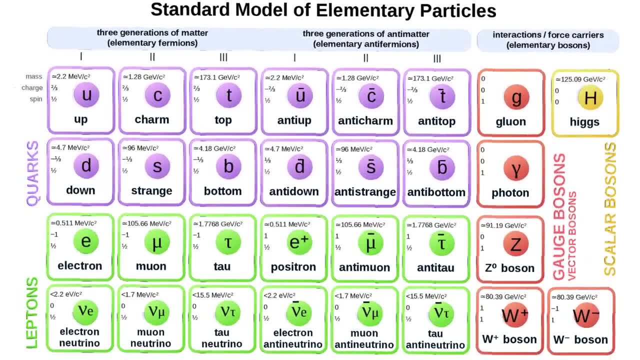 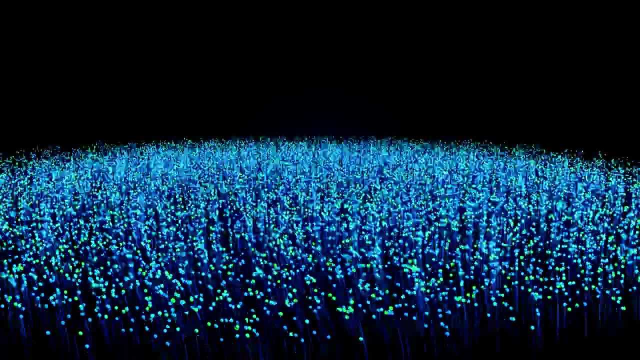 antiparticle. The antiparticle has the same mass and spin, but possess opposite charges and other quantum numbers compared to their corresponding particles. However, it is important to note that matter cannot be built from both particles and antiparticles. When a particle encounters. 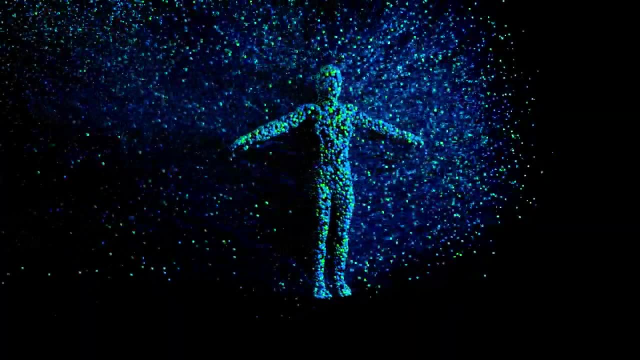 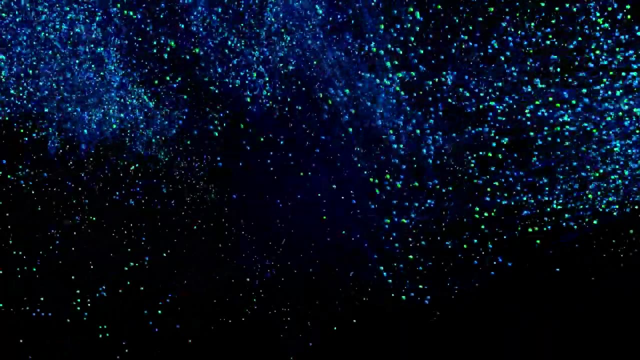 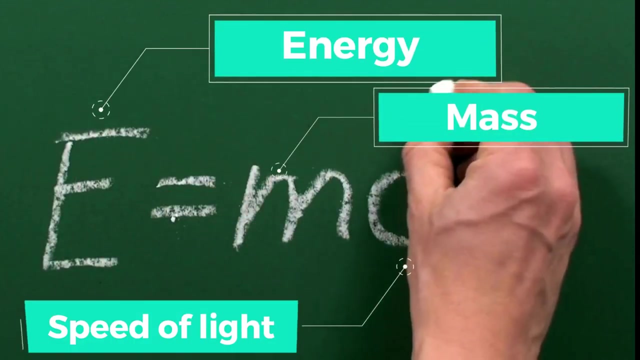 its corresponding antiparticle. they annihilate each other in a process known as annihilation During annihilation. the total mass of the particle-antiparticle pair is converted into energy in accordance with Einstein's famous equation: E equals mc- c squared, where e represents energy, m denotes mass and c is the speed of light In the everyday. 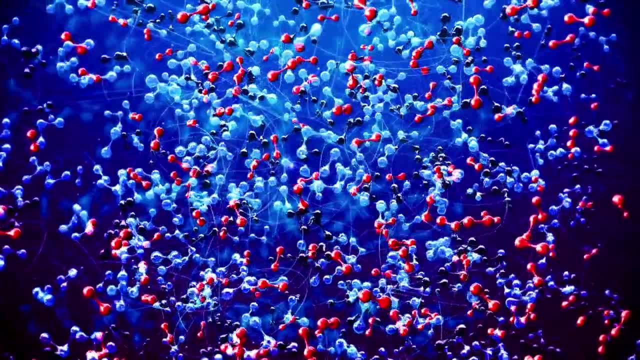 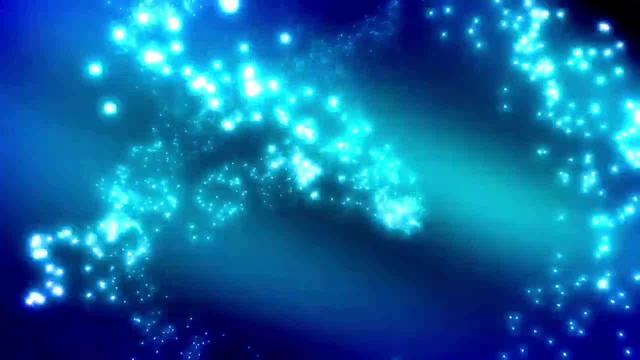 world, there is an excess of electrons, protons and neutrons compared to their corresponding antiparticles- positrons, antiprotons and antineutrons. The absence of significant amounts of antiparticles in normal matter allows for the formation and stability of atoms, as well as the 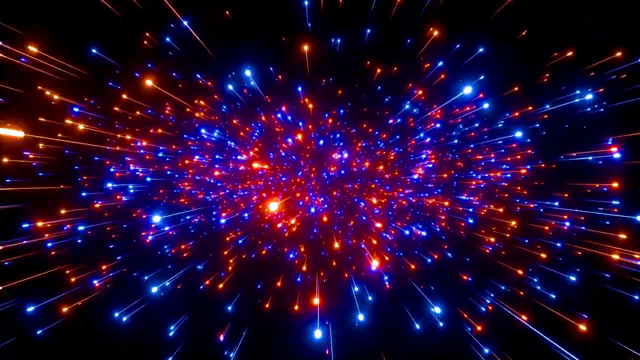 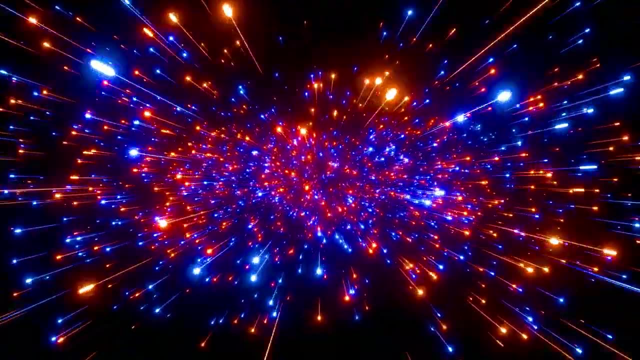 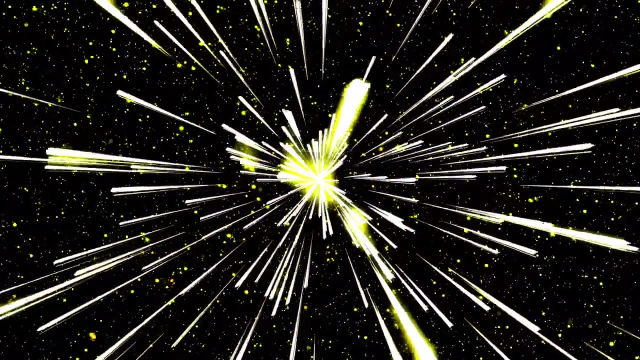 complex structures that constitute our everyday world. Natural positrons do indeed exist, and they are created through high-energy cosmic rays that originate from outer space and interact with particles in Earth's atmosphere. Cosmic rays consist of energetic subatomic particles, such as protons and other atomic nuclei that travel at significant speeds. When cosmic rays 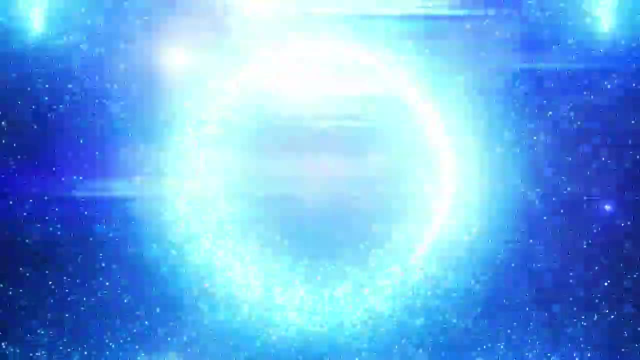 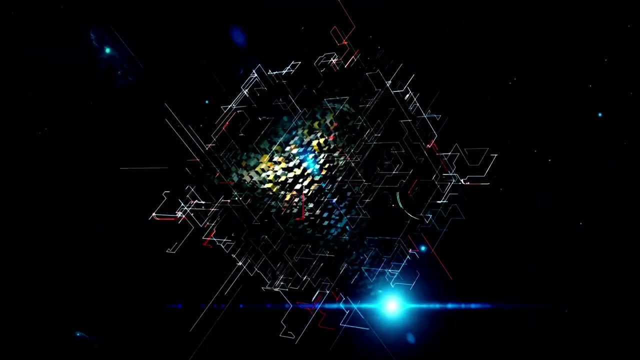 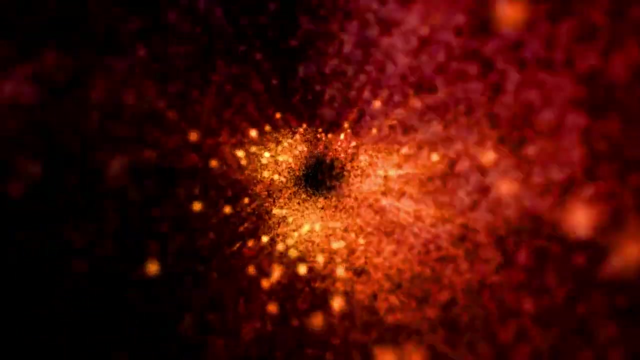 collide with atomic nuclei in the atmosphere, they generate extensive particle showers. The immense energy carried by the cosmic ray is transformed into various forms of matter. in accordance with Einstein's theory of special relativity, e equals m c squared and e equals m- c squared. Among the particles produced in these cosmic ray showers are pairs of: 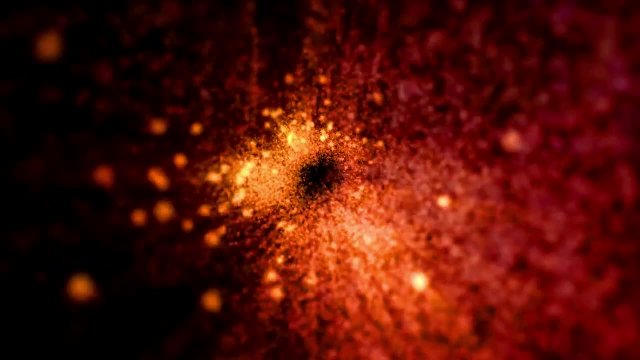 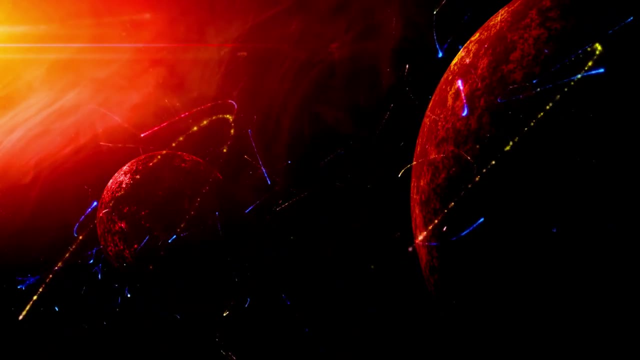 electrons and positrons. These electron-positron pairs are created due to high-energy interactions and conservation laws. However, positrons have a very short lifespan and survive for only a fraction of a second before they encounter electrons. When a positron and an electron come close to each other. 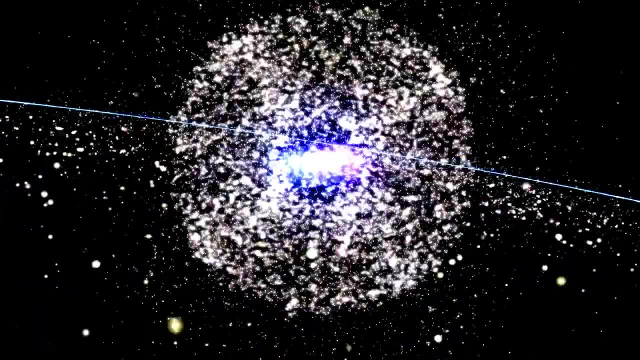 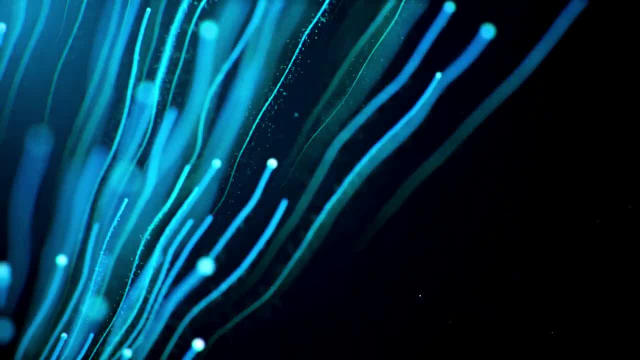 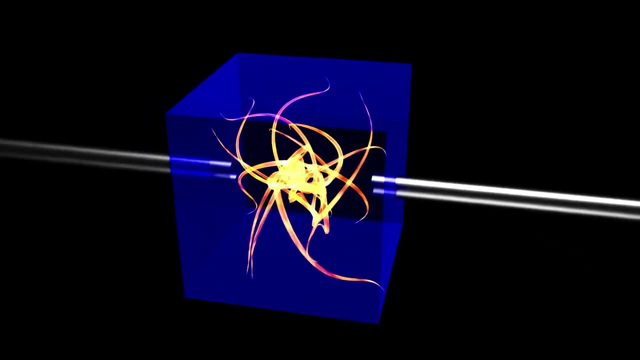 they annihilate, resulting in the complete conversion of their combined mass into energy. In particle accelerators, physicists are able to recreate high-energy collisions that mimic the interactions occurring in cosmic rays. In 1955,, a significant breakthrough occurred in the field of particle physics when a team led by 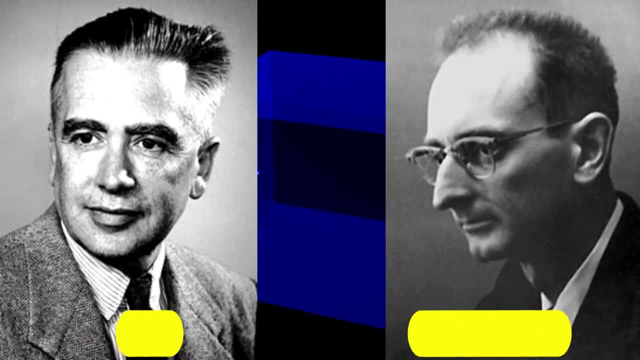 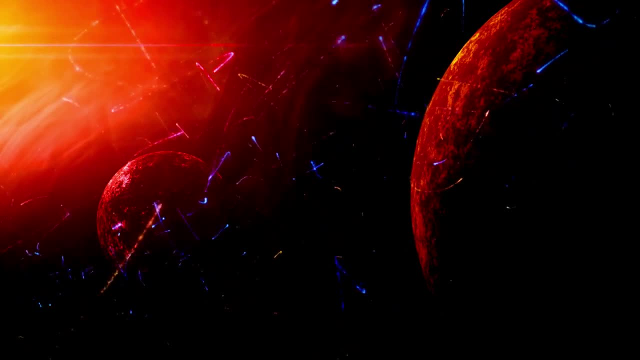 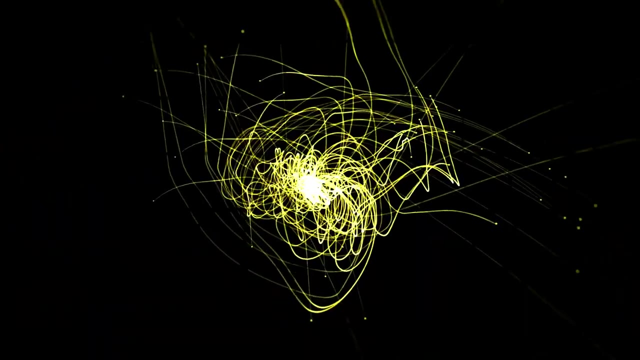 Emilio Segri and Owen Chamberlain conducted experiments at the Bevatron, an accelerator located at what is now the Lawrence Berkeley National Laboratory in California. They were searching for evidence of antiparticles, specifically antiprotons. The experiment involved colliding high-energy protons with target atoms. In these collisions, 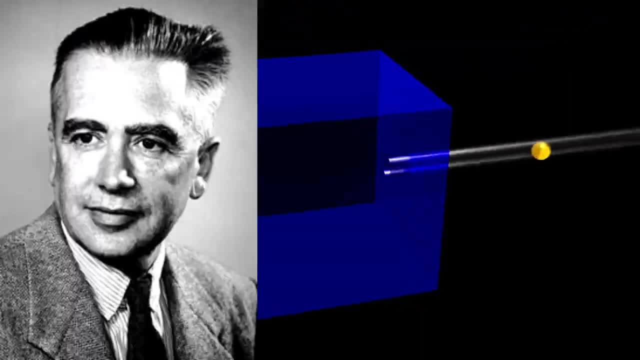 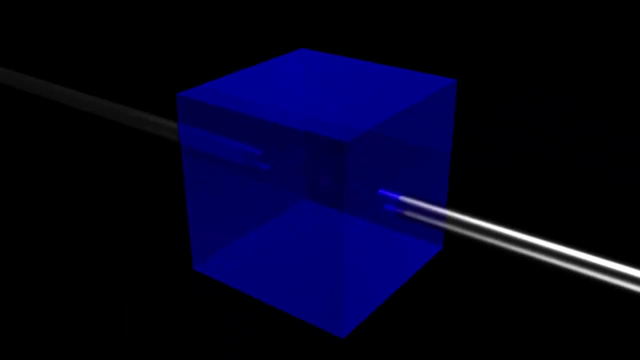 some of the energy was converted into a particle and some of the energy was converted into a particle. Segri and Chamberlain's team observed the creation of particles with the same mass as protons but with opposite electric charges. These particles were identified as antiprotons. 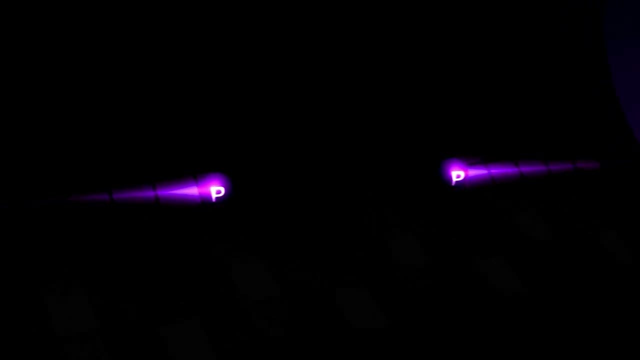 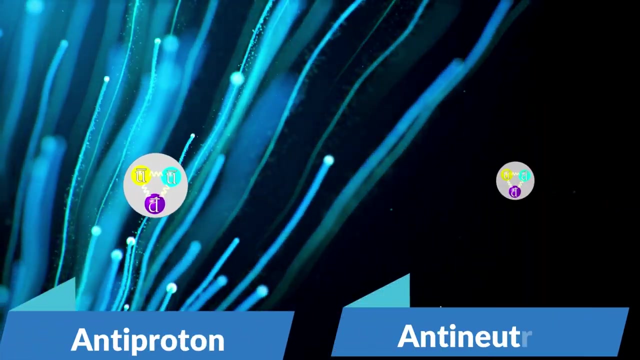 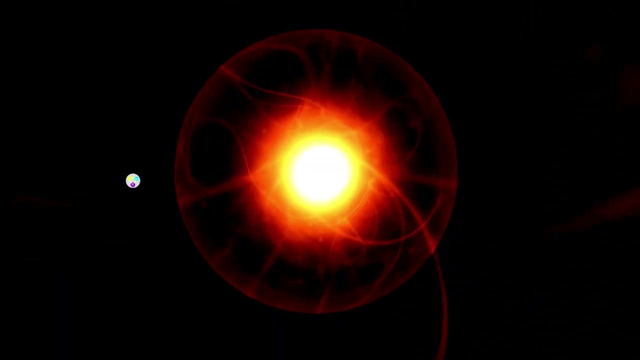 the antimatter counterparts of protons. Shortly after the discovery of antiprotons, another team working at the Bevatron discovered the antineutron. The discoveries of antiprotons and antineutrons in particle accelerator experiments provided experimental confirmation of the existence of antimatter. Since the discovery of antiprotons, 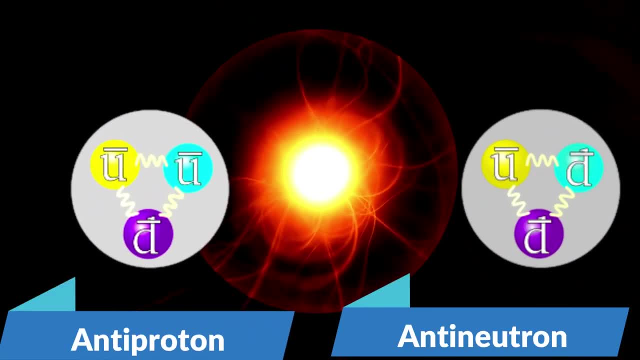 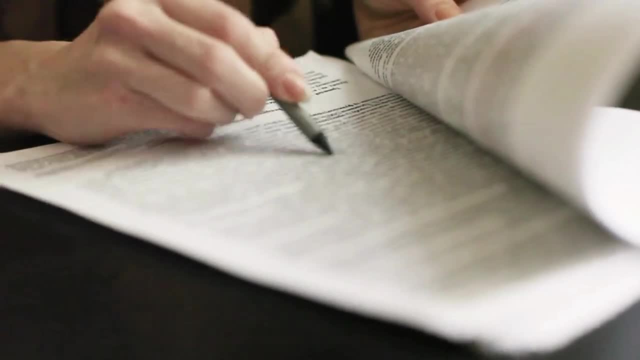 protons and antineutrons in the 1950s, physicists have made further progress in understanding the fundamental particles that make up matter. Since the 1960s. studies have revealed that protons and neutrons, which were previously considered elementary particles, are composed. 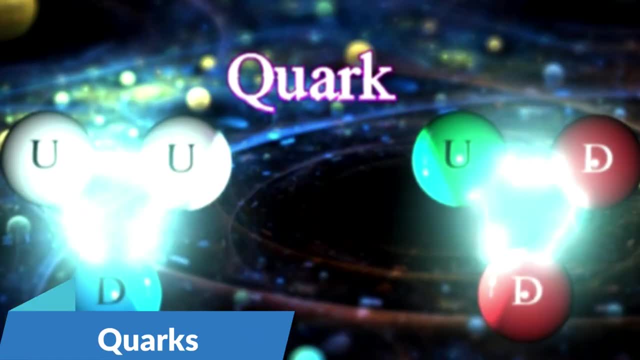 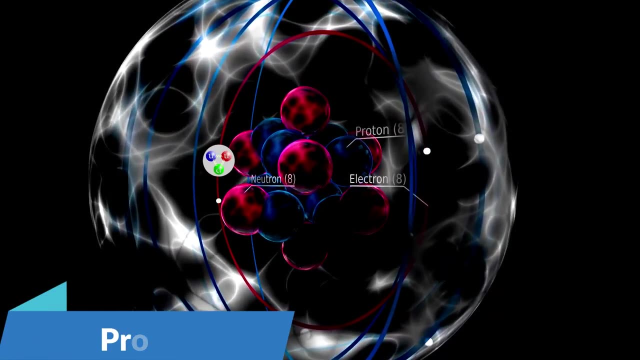 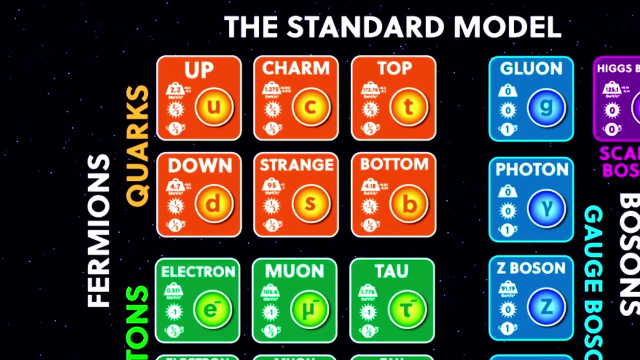 of even smaller particles called quarks. Quarks are point-like particles with fractional electric charges and a property called spin, which determines their intrinsic angular momentum. Protons and neutrons are composed of three quarks each. The combination of different types of quarks gives rise to the different properties and behaviors of these particles. 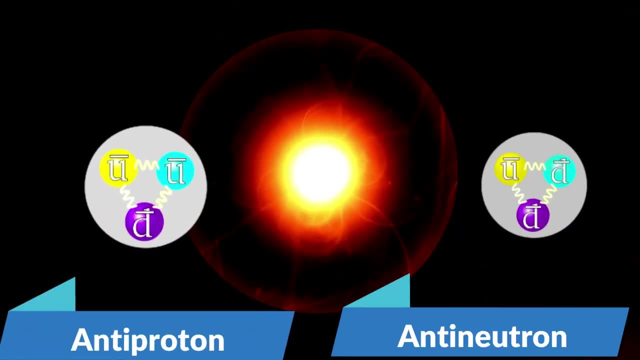 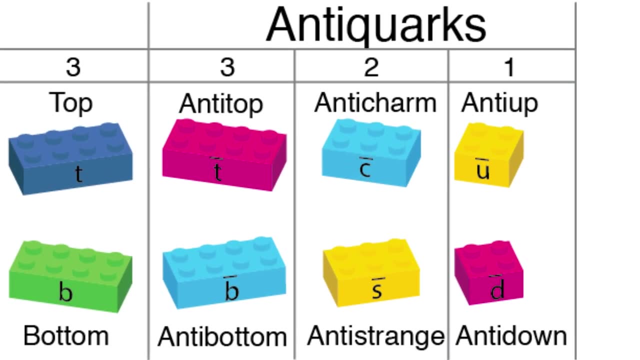 Similarly, antiprotons and antineutrons are composed of antiquarks, which are the antiparticles of quarks. Antiquarks have opposite electric charges compared to quarks and exhibit the same fractional spin. Neutrinos, on the other hand, are elusive particles with very 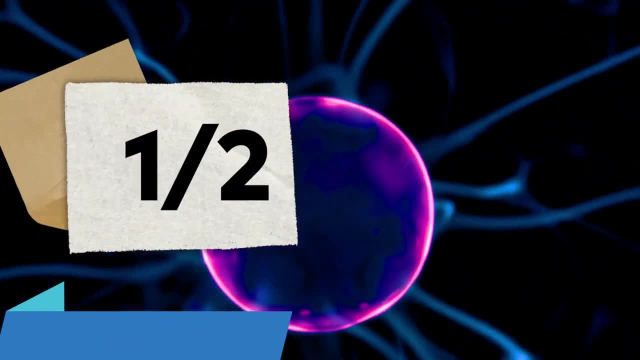 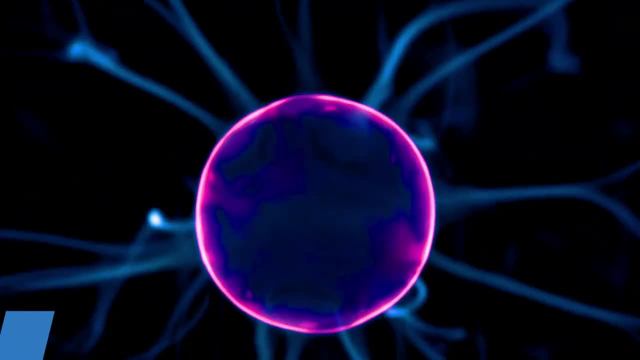 little mass and no electric charge. They also possess spin of one-half. Just like quarks, neutrinos have corresponding antiparticles, known as antineutrinos, which have opposite properties. The understanding of particle interactions and decays led to the realization. 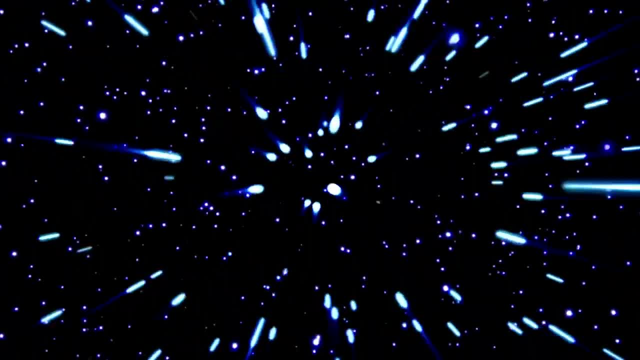 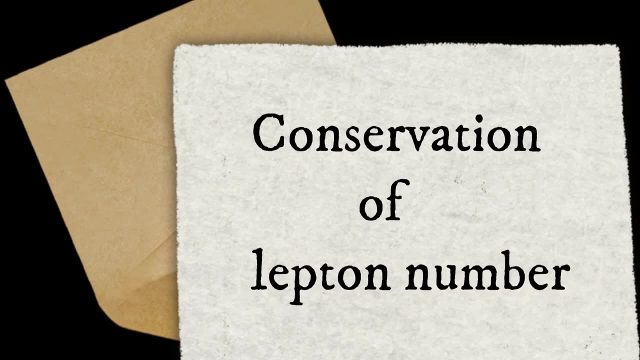 that certain conservation laws govern the behavior of quarks and leptons, particles like electrons and neutrinos. One such law is the conservation of lepton number, which states that the total number of leptons minus the total number of antileptons remains constant in any interaction. 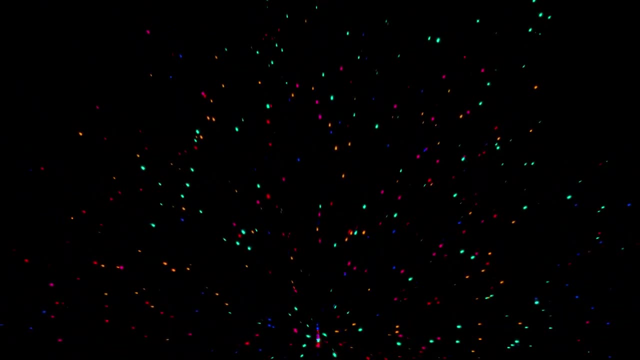 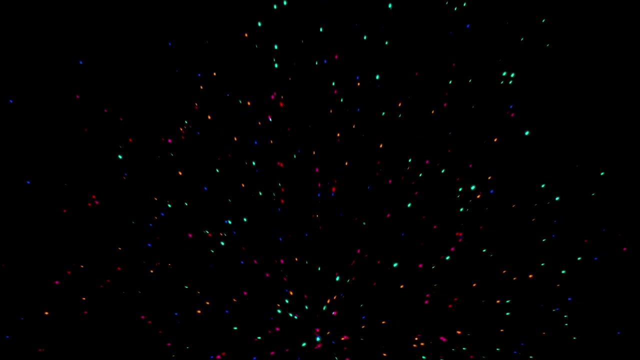 This means that if a lepton, such as an electron, is produced in a decay process, an antilepton- in this case an antineutrino- must also be produced to balance the lepton number, In addition to the familiar particles like protons, neutrons and electrons. 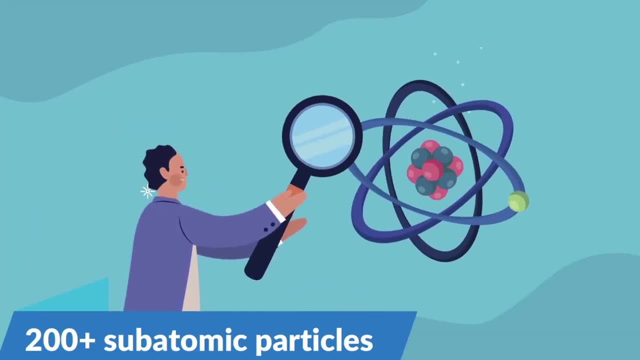 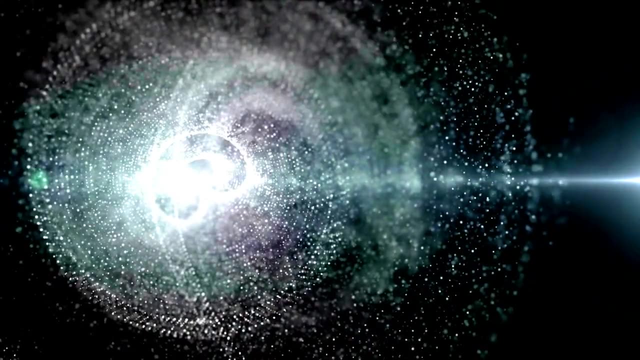 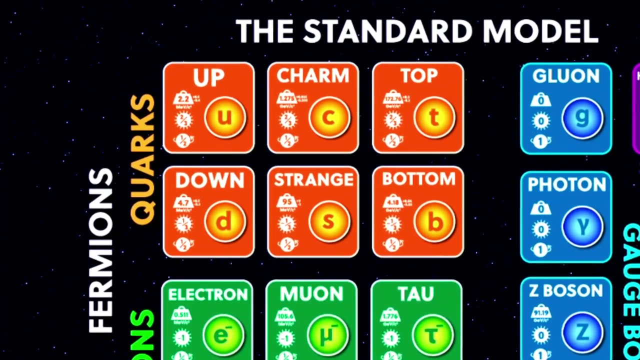 scientists have discovered the existence of more than 200 other subatomic particles. These particles, often referred to as extra particles, are not commonly observed in everyday low-energy environments, but emerge under the higher energies found in cosmic rays or particle accelerators. The behavior and variety of these additional particles have been explained through. 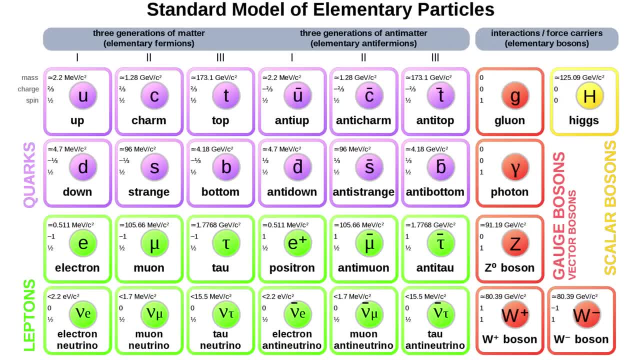 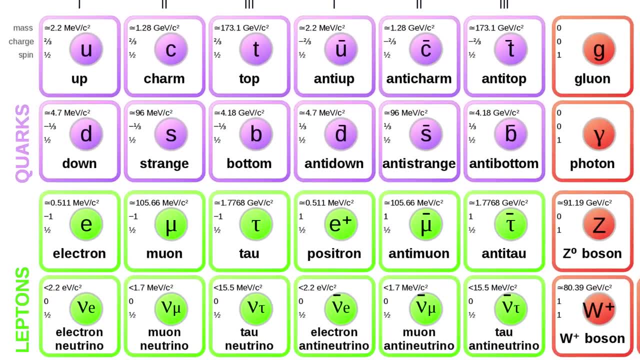 the framework of the Leibniz-Leibniz-Leibniz-Leibniz-Leibniz, The framework of quarks and leptons, which are fermions, With just six types of quarks and six types of leptons, along with their corresponding antiparticles. physicists can account for the.